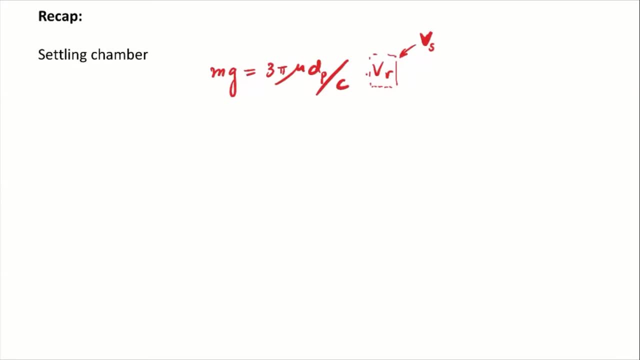 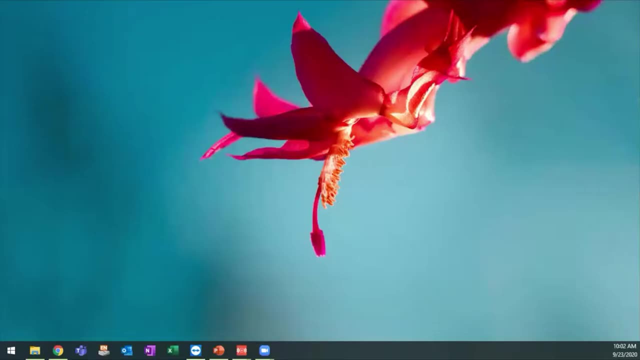 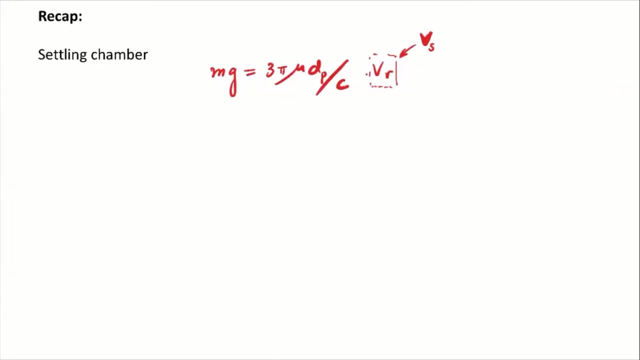 removal efficiency. so here I think we can spend some time to do a quick quiz about calculation of the of the particle removal efficiency. see here, set it up. all right, so it's a simple calculation here. let's spend maybe one or two minutes to work on this right. 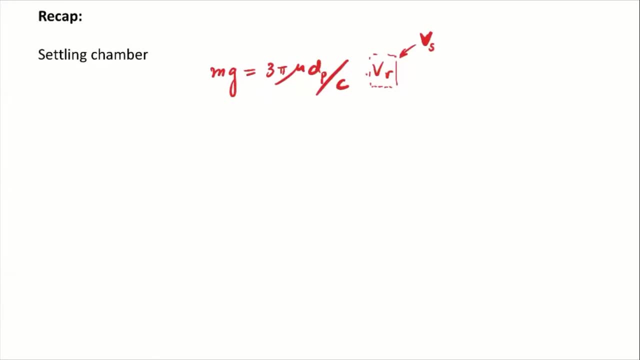 so basically it's saying that in a settling chamber we have particles of two different sizes because the smaller sized particles have a lower gravity, right so the removal efficiency is lower. well for the head of the particle. we have a lower gravity, right so the removal efficiency is lower. well for the head. 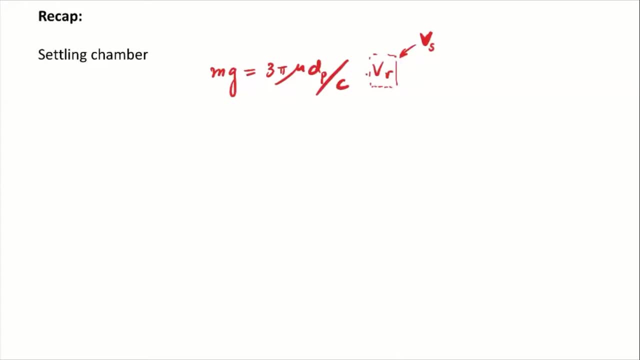 of your particles, the removal efficiency is higher. you can take your time, maybe spend two minutes or three minutes on this. I think most of you have got an answer. you can take your time, maybe spend two minutes on this. I think most of you have got an answer. 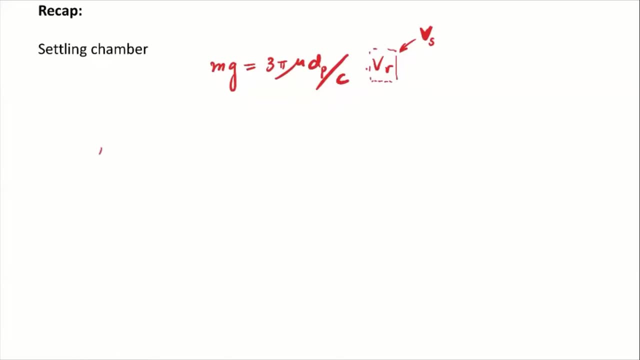 so remember, when we calculate the removal efficiency specifically for the two different sizes, we've mentioned that it can be calculated by m 1 plus m 2 on the denominator m1e, practicallyева one in the denominator m1 in the denominator m1e. 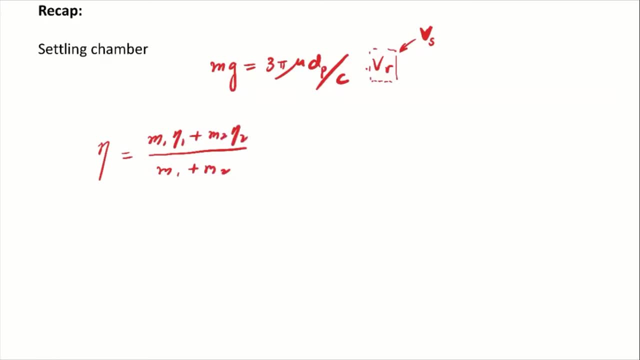 right, this is not blocking the equation. okay, ten more seconds. okay, we'll stop here. I think just have one student who didn't submit the answer, so most of you guys are correct. it should be 50%. so basically we just plug in the mass concentrations, right? so it's 100 here in the 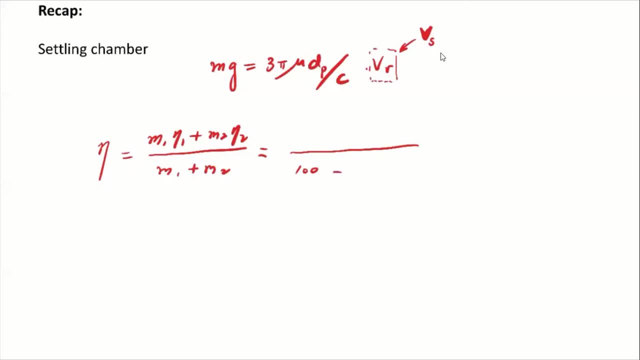 denominator, basically 100 plus 100, then 100 multiplied by 30 percent, and then 100 multiplied by 60- 70 percent, right? so finally you get 50 percent in terms of overall particle removal efficiency. so I would say that this setting here is a little bit it's. 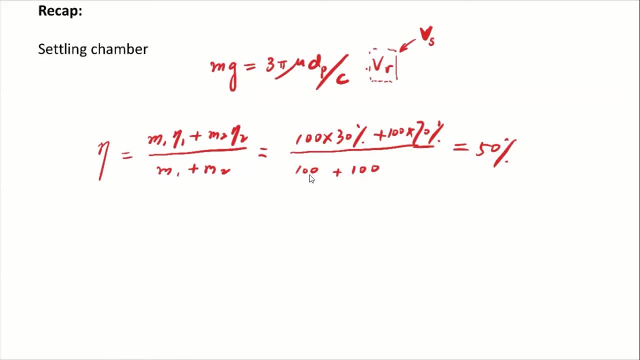 quite straightforward, right? so basically you have both concentrations at 100. let's say, if we change one of the concentration to 50 microgram per meter cube, then you also have to change that in here, right? so the answer will be quite different. so basically, it's not 100 percent, right? so? because you're not 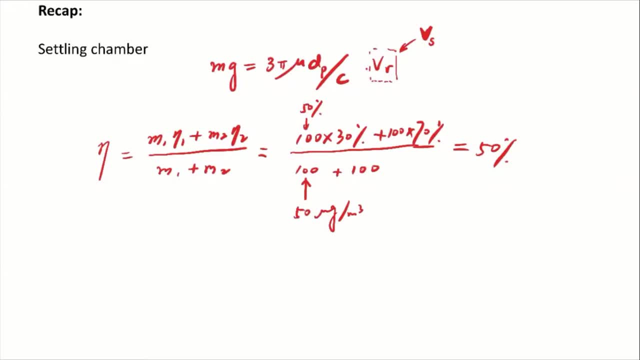 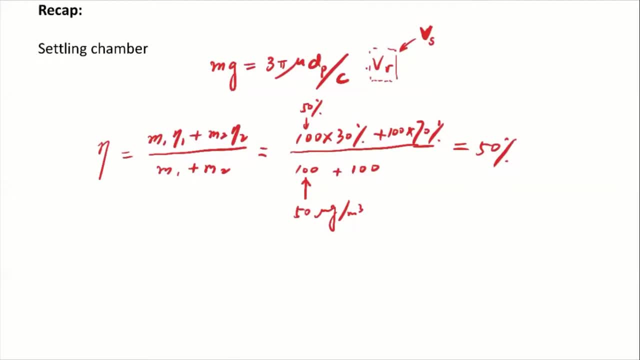 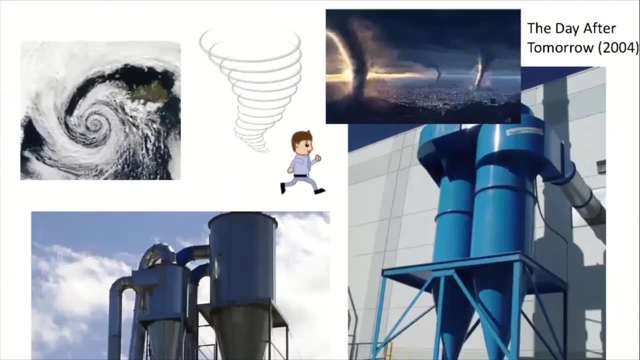 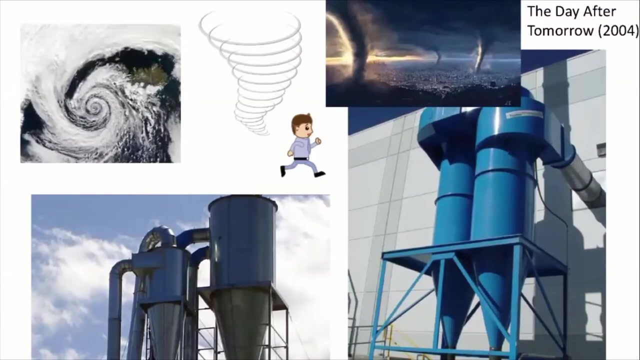 the calculation of the cycle, you'll get more understanding regarding this overall removal efficiency. all right, so now let's start with the new contents. okay, so here I'm showing a few pictures of the cyclones. so whenever we mention cyclones, say it's something similar to tornado, hurricane or typhoon, depends on. 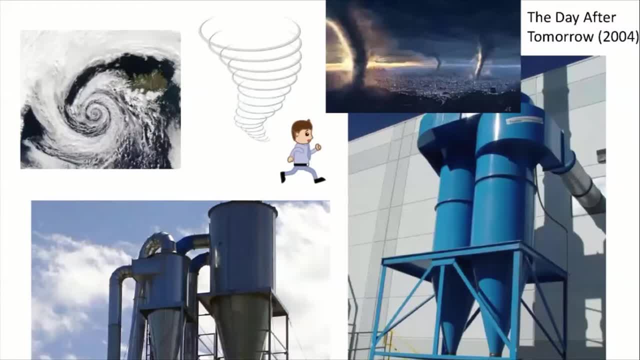 where, where you live in, people have different names for these rotating systems, right? so typically the air, let's say the air- will rotate inside right and will form these rotational movement of the air flow. so I'm not sure if you have seen a typhoon or seeing a cyclone. very 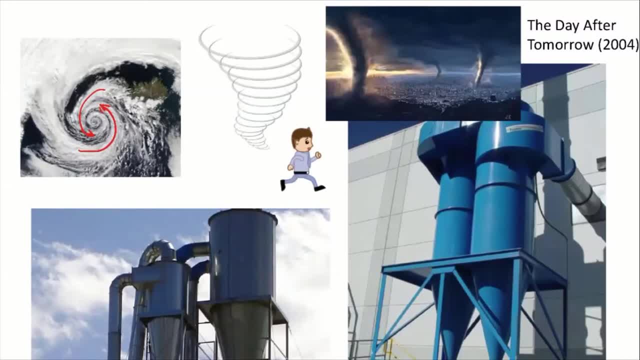 in close distance. I have never done that. I think it's it should be quite dangerous, right so, but I'm pretty sure that we have watched it on movies or on TVs. I know that there are people- you see the weather channel. there are people chasing the cyclones and they're chasing the cyclones and they're chasing the. 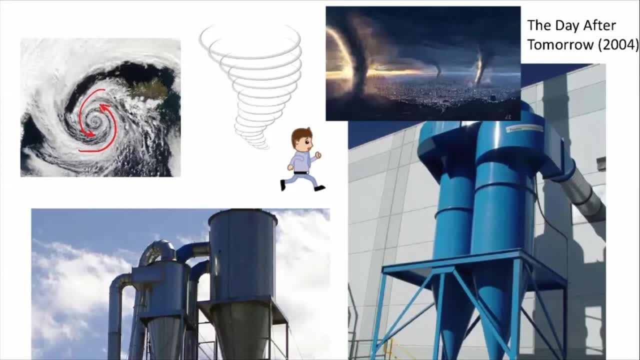 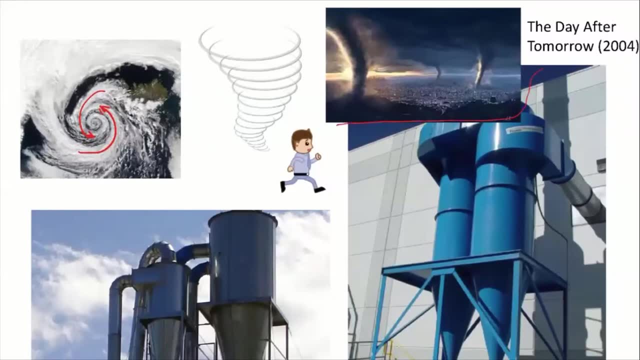 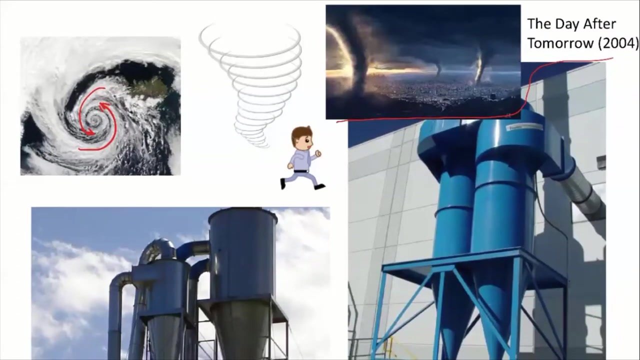 tornadoes, chasing the hurricanes, right. so here I'm just showing a screenshot of a movie. I like this movie quite a lot. it's the day after tomorrow, it's about climate change and some science fiction, right, and although it has a pretty low rating- and I don't know what's the reason, but I think it's quite amazing to. 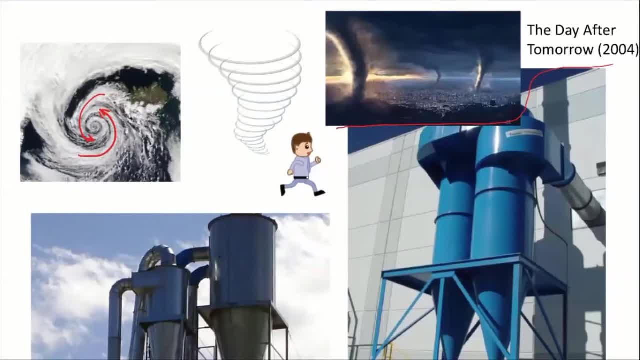 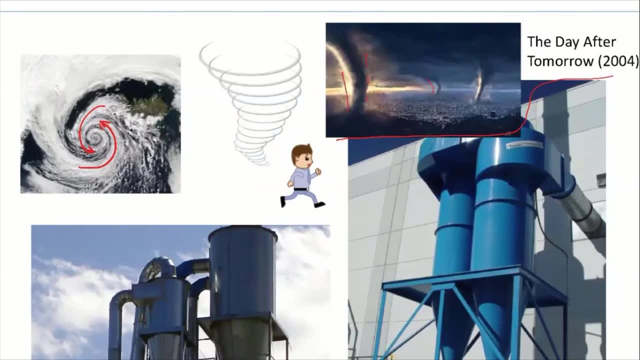 show what is the impact of the climate change, right? so there are a lot of people that are watching this video and there is a lot of information about the weather. so you can go to the Google map and you can see that they're showing several hurricanes or several tornadoes just over the cities, right? so if you 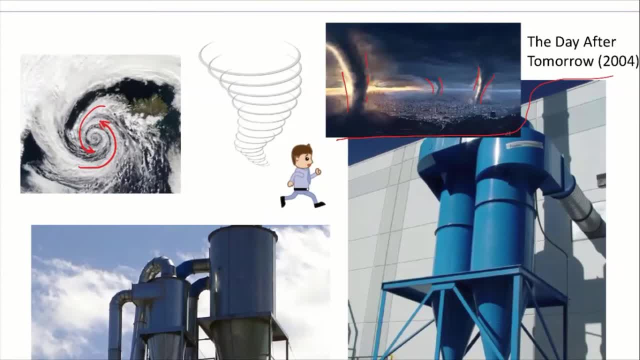 basically, if you watch those, those videos, you can see that typically the larger objects will get spinned out, right? so I had the impression that some particles or larger objects will just get spinned outside. It's similar to the washing machine that we use, right, The high speed of water is spinned out. 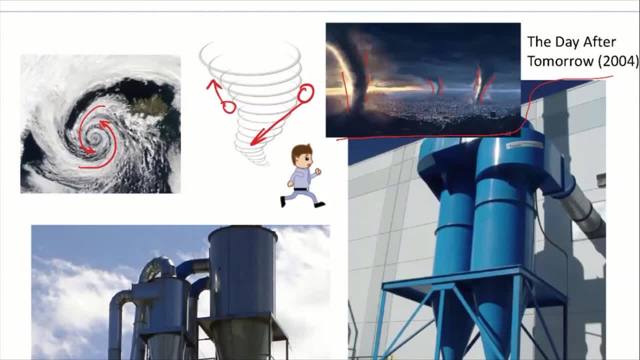 So the reason why these larger objects can spin out and can get spinned out is because of the force balance. So we know that if any object wants to do this rotational movement, they have to have a centrifugal force. Basically, a force has to support the particle to rotate or the object to rotate around the 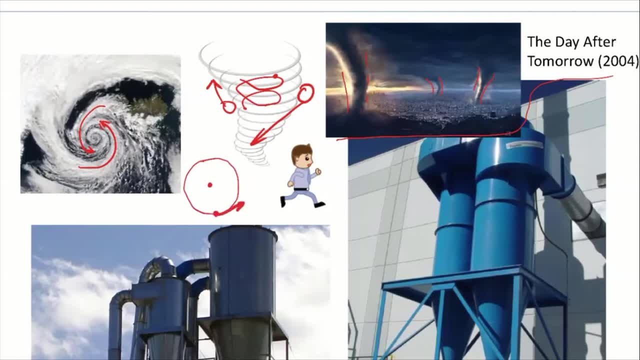 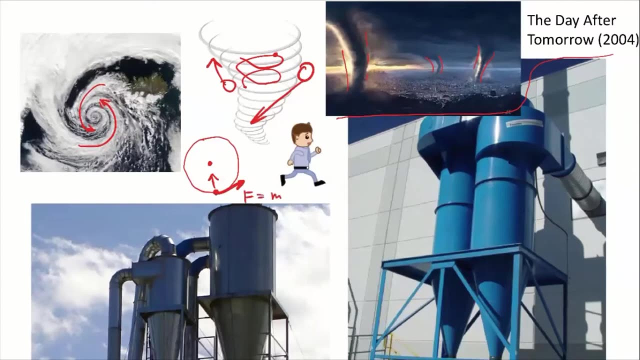 center. So, for example, if an object rotates in this way, then there should be a force that's providing this centrifugal force. right So, for these larger objects, because they're so large, we know that centrifugal force is basically F equal to MV squared divided by R. right So, at the same, 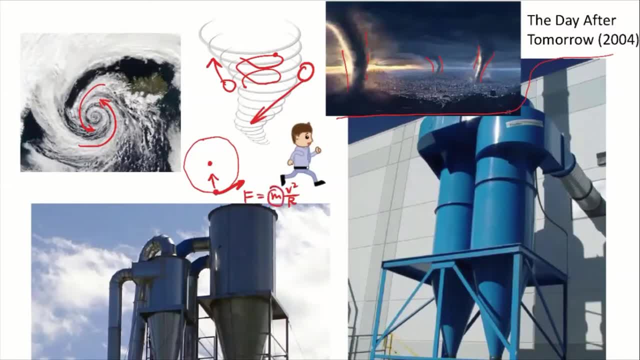 velocity and same radius. the heavier the object, the larger the centrifugal force. So basically, these larger objects, they don't have enough of a force to support that centrifugal force, So that's why they will be the rotational movement. They will leave the cyclone here right. So we can use the same mechanism to 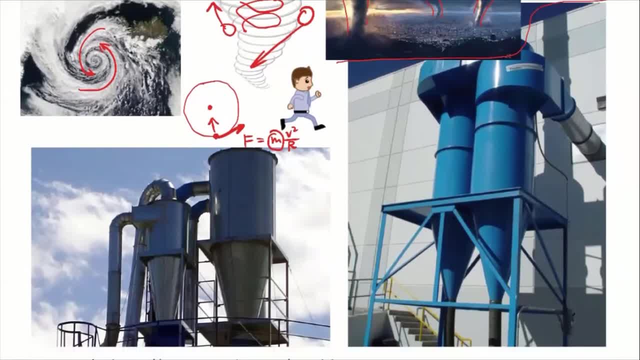 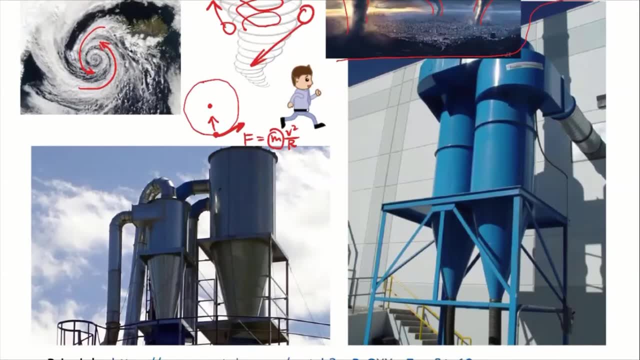 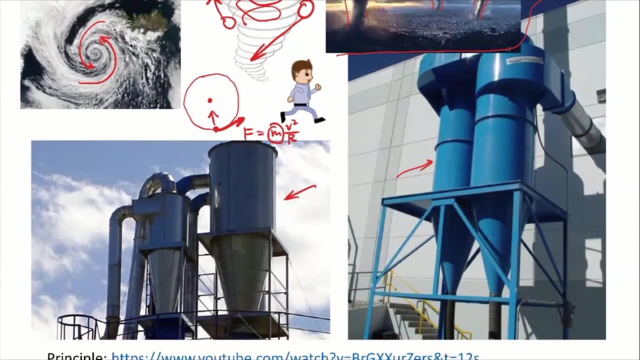 remove particles. So I'm not sure if you go to- you have been to- some industrial plants or power plants, So there you can typically show. if you go to a power plant you can typically see these devices, These ones. So it's mainly 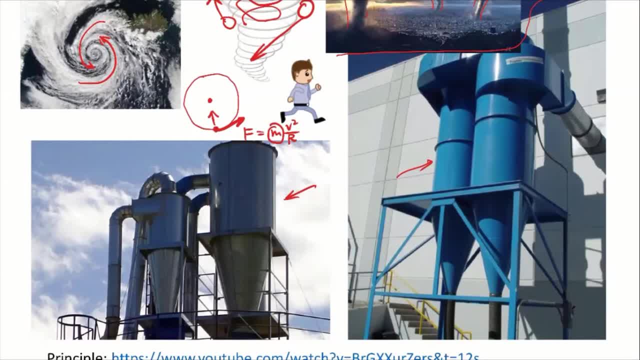 composed of a cylinder that's at the top, and then you have a cone at the bottom. Okay, So what happens is that the air will enter from the side of the cyclone, So this is called a cyclone. You enter from the side of it and then get. 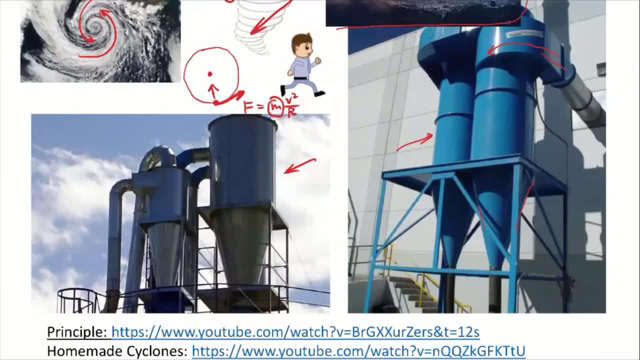 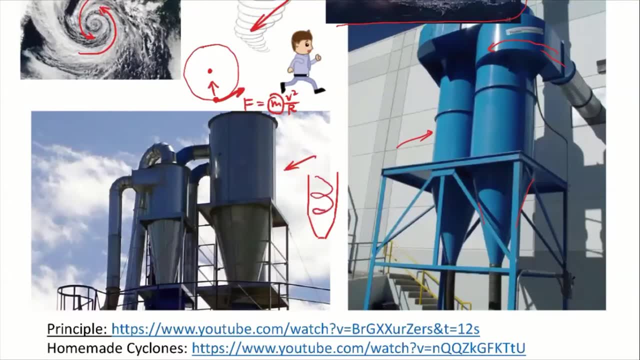 introduced into this cylinder. So what happens is the air is going to- let's say The air is going to- rotate, right. So the heavier particles, or the larger particles, because they don't have enough of a force to support the rotational movement, they will just get spinned onto the wall. 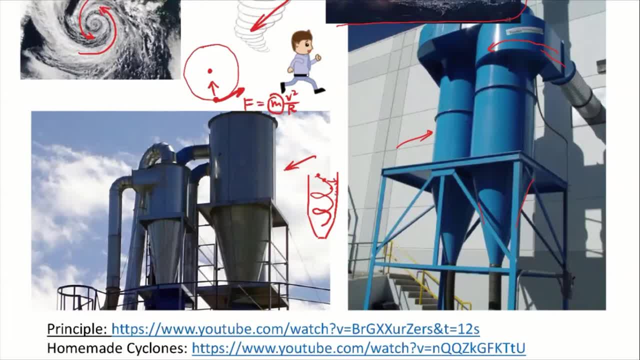 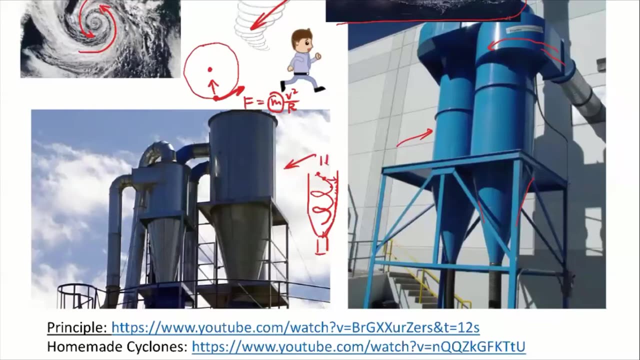 On the wall, you will collect larger particles and then, because of gravity, they will just fall down along the wall and then finally get collected. at the bottom, right- And for these devices, typically at the top, there's also an outlet, okay. 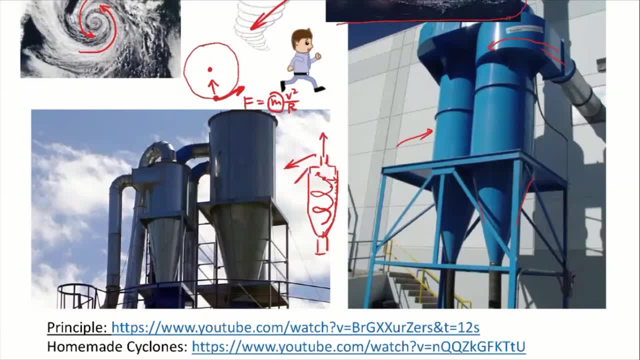 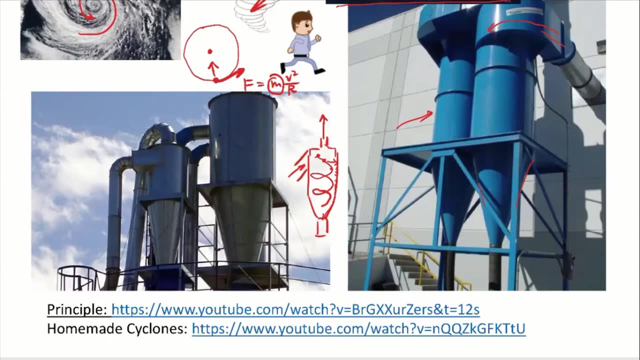 So the outlet will draw the air flow outside. So we mentioned that the air will enter from the side and then get drawn outside. okay, So in this way we can basically introduce particles into the system and then withdraw the remaining air flow from the system. 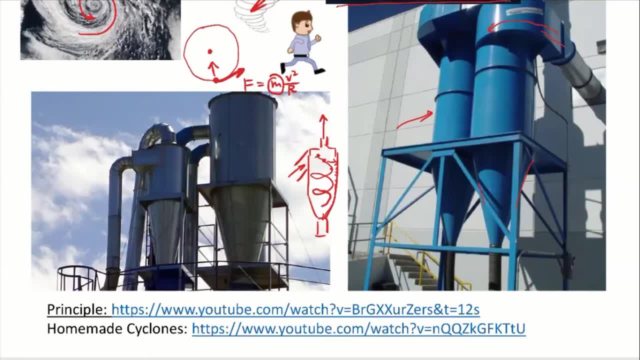 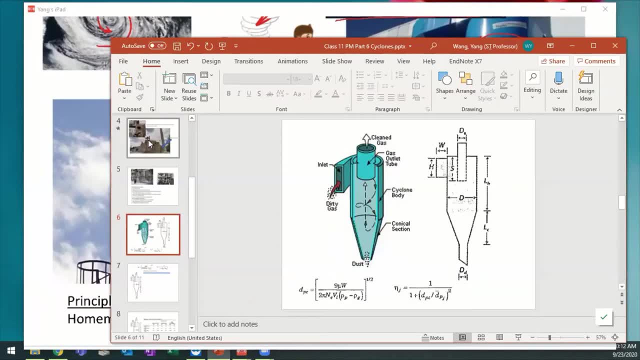 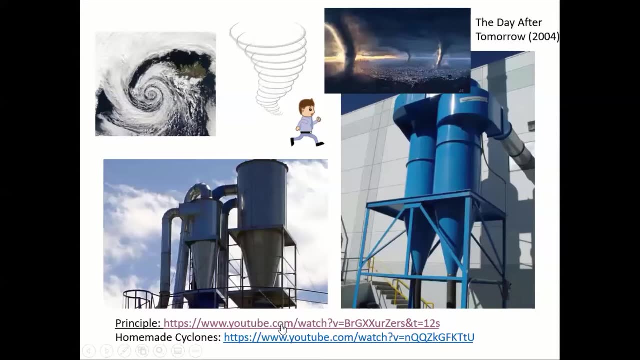 So there's a mass balance of the air flow, All right, So here I can basically show you a video about the working principle of the cycle. Let's do this. So can you hear the – yeah, maybe not, yet Let me do this. 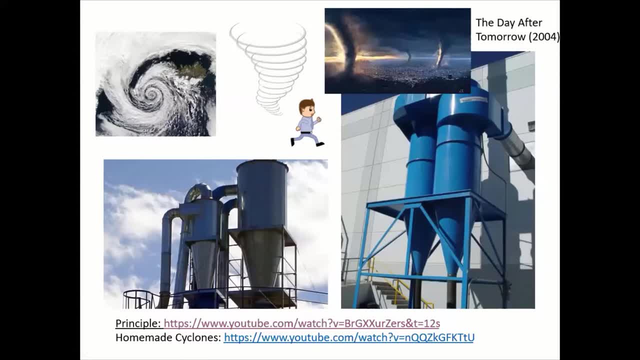 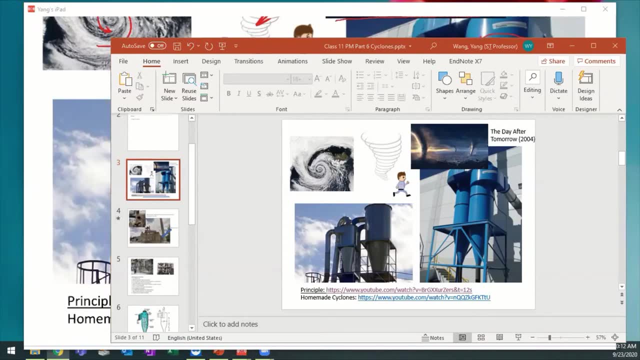 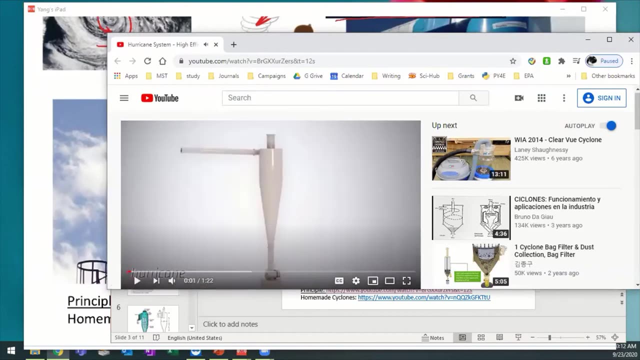 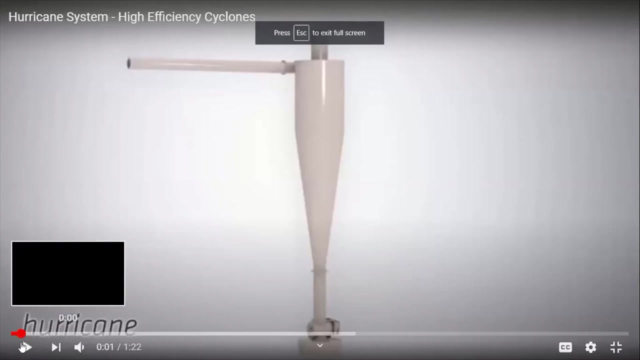 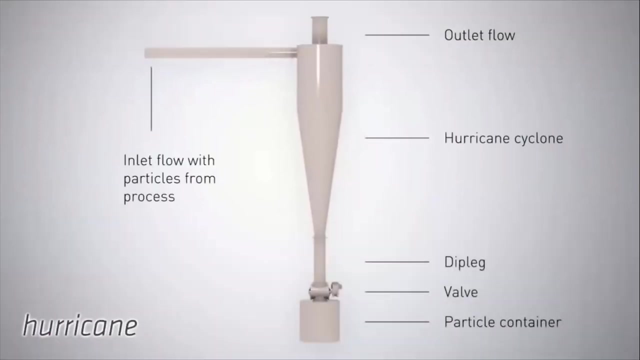 Let's see. All right, so you can see the video here, right, Okay, All right, So you can see the video here, right, All right? hurricanes are customized cyclones to serve different needs and which results from optimization functions such as maximize efficiency, minimize cost or minimize size, combining stochastic. 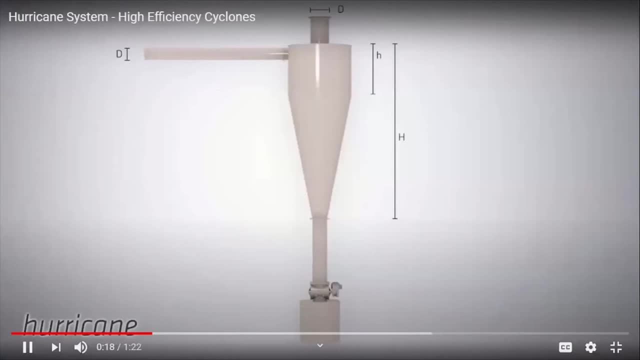 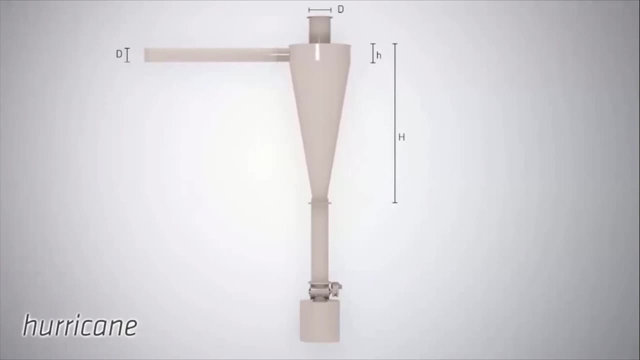 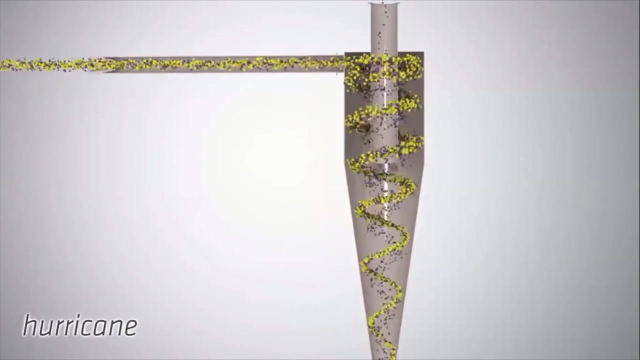 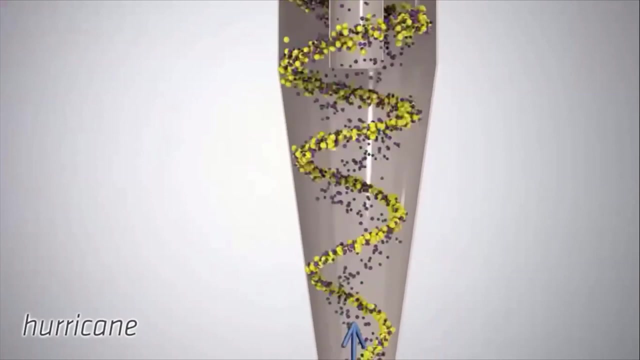 numerical optimization by changing the eight independent cyclone dimensions. with the knowledge of particle agglomeration, ACS is able to design the perfect geometry for each case. the colored dots indicate the particulates to be collected and the blue arrow represents the flow of gas that leaves the equipment for dusts with tendency to agglomerate, such as biomass or coal fly ash. 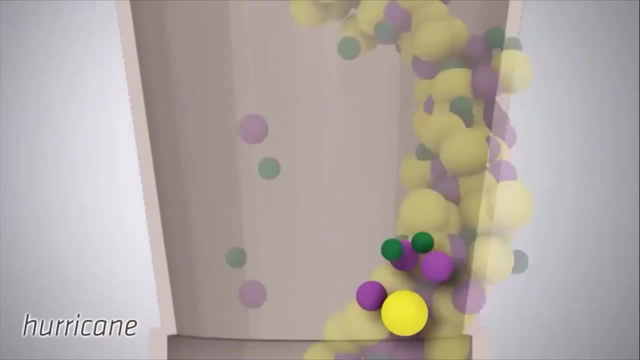 among others. efficiency is maximized thanks to the clustering effects of particles. in fact, the cyclone doesn't see as many swathes of particles as it does. the cyclone doesn't see as many swathes of particles. in fact, the cyclone doesn't see as many swathes of particles. in fact, the cyclone. 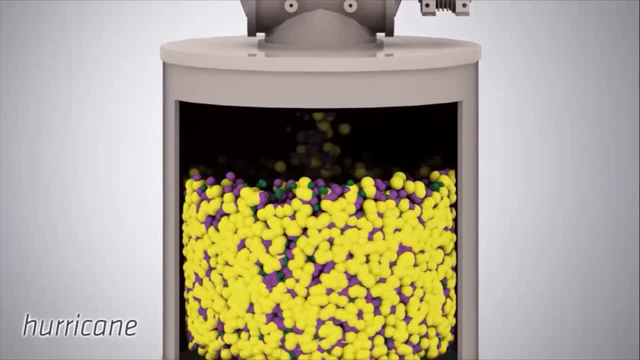 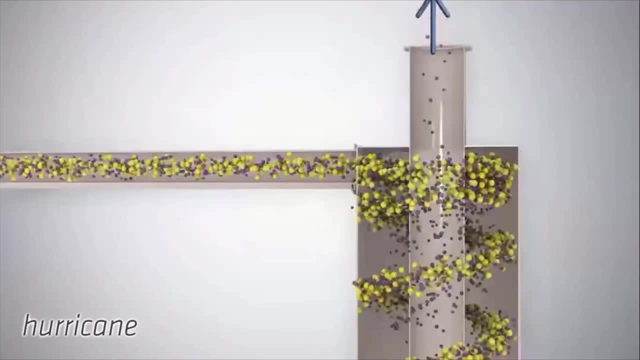 doesn't see as many swathes of particles. in fact, the cyclone doesn't see as many swathes of particles, but clustered particles with bigger dimensions, thus easier to collect. agglomeration increases with wide particle size distributions, long residence times in the cyclone and large inlet. 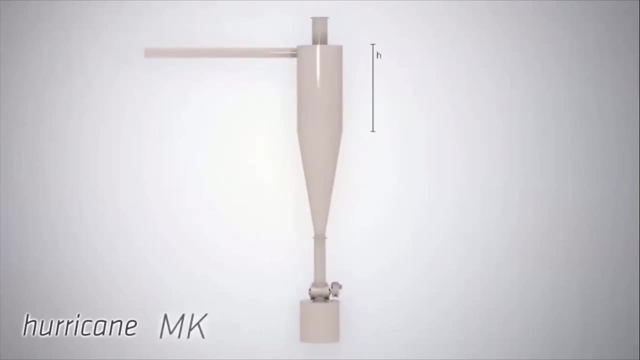 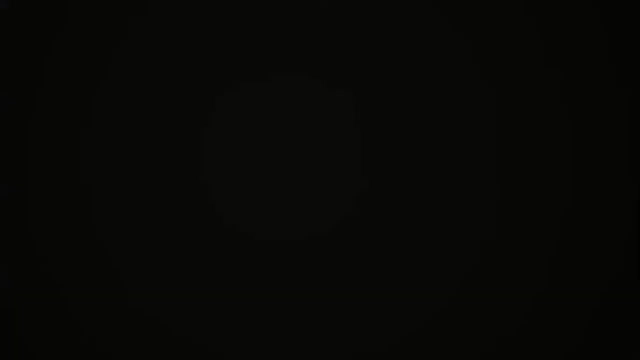 particle concentrations. agglomeration is maximized with the new developed hurricane mk. cyclones emissions can be under 15% of those of other cyclones, being as low as 30 milligrams a normal cubic meter for many industrial products. the paper does notó. 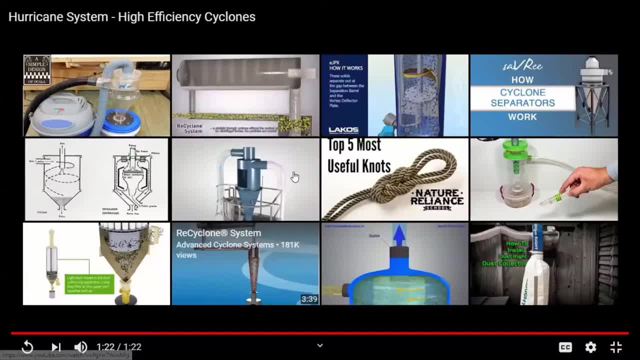 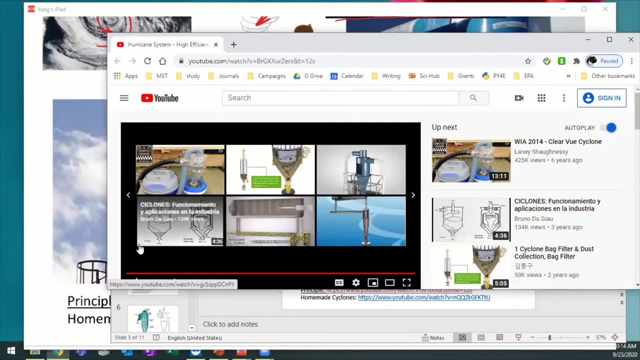 vor of the hunger in a cyclone, an autonomous vehicle, Tilithien. okay, so this is a commercial for a cyclone system and they call it Hurricane or hurricane or tornado or typhoon. so basically they are in general industry we'll call them as cyclones. 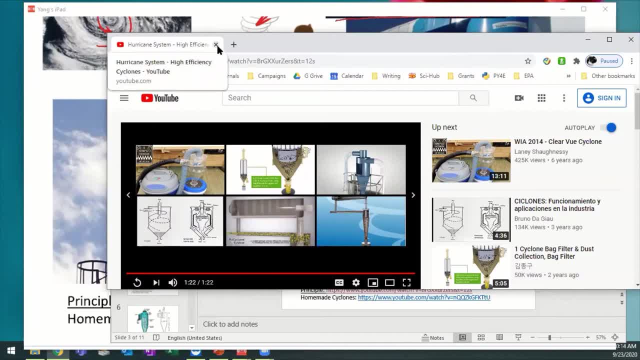 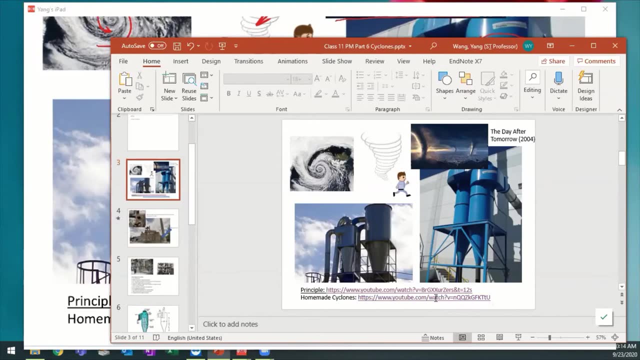 okay, we see that the major mechanism is that the larger particles, because of their larger mass, they'll get spent outside, right, so finally you can. so there's also quite interesting video about a homemade cyclone. So if you have a, have a vacuum at home so you can. 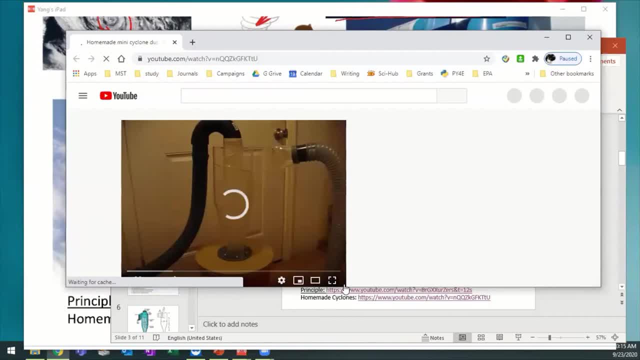 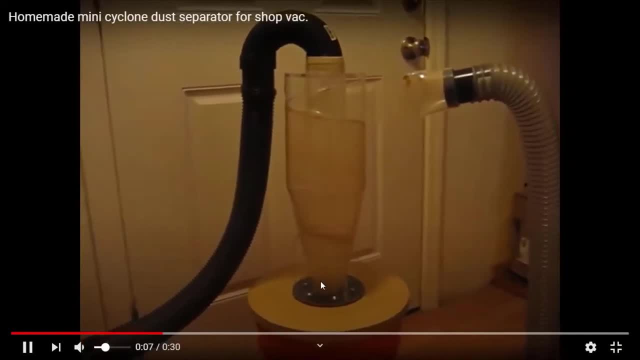 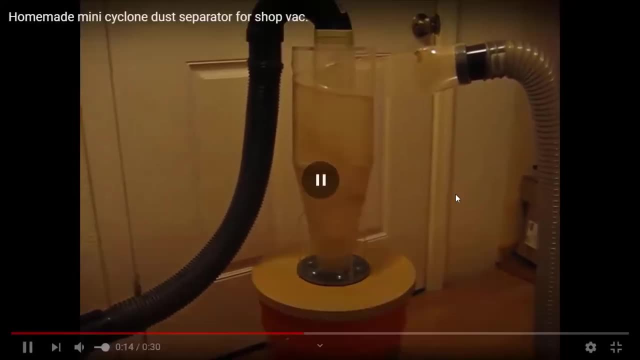 actually make this one. Yeah, you see, the air flow, the particles, So there's actually a quite interesting phenomenon. So, you see, when the air draws the inside, it actually flows like a band, right, because air is incompressible. 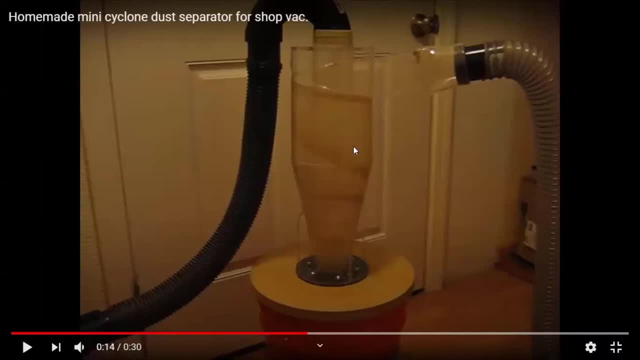 So they flow like a, like a ribbon, and then they just stack on each other right. then, finally, when they get to the get to the bottom, where there's a cone, they have to get compressed and then this is outlet, So the air is withdrawn. 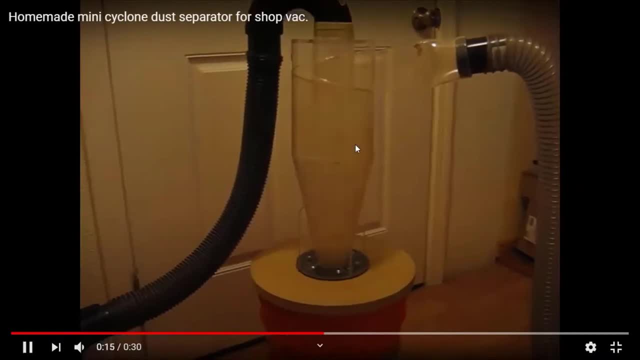 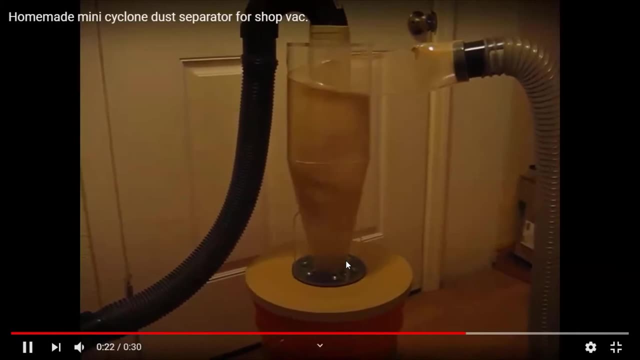 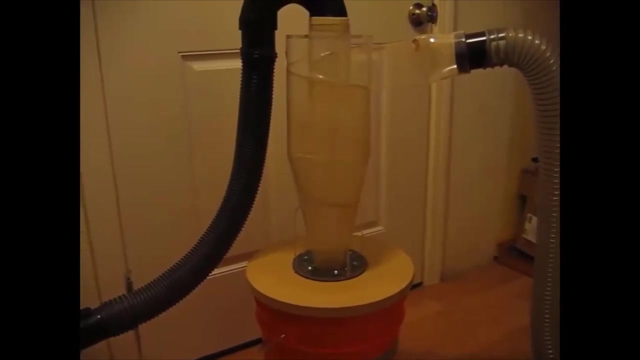 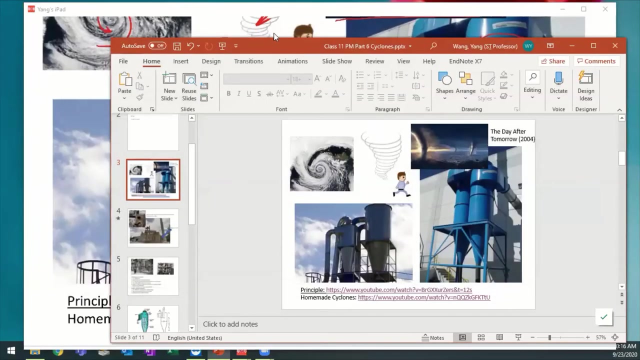 from the top. You can see how the air flows from the top to the bottom of the cyclone, and then you can see how the air flows from the top to the bottom of the cyclone. So this is the basic principle of a cyclone. Let's get back here. 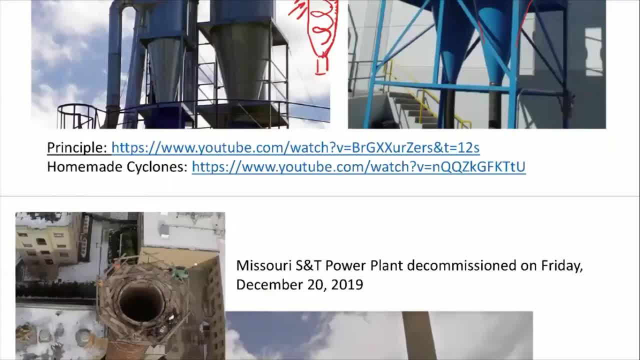 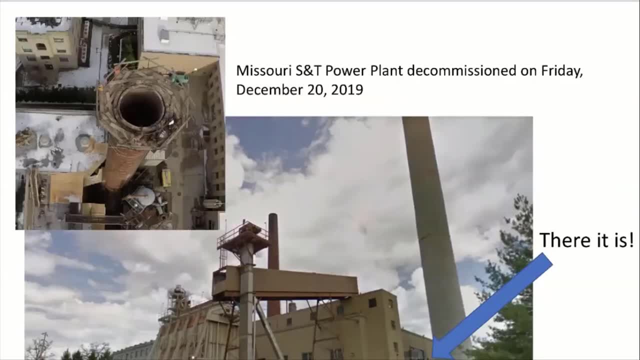 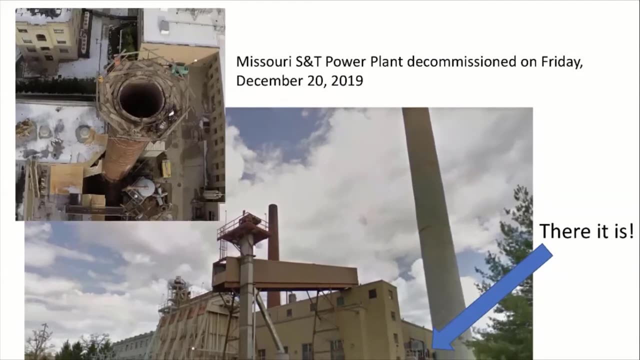 So I think maybe most of you know that our school used to have a coal-fired power plant. So last year, actually last December, so our school decided to decommission the power plant right. So I was a little bit upset about that, because whenever I 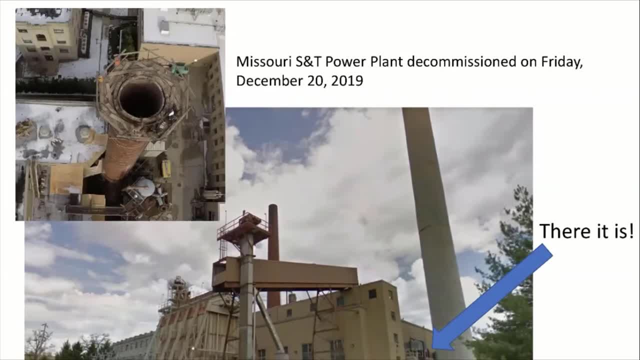 teach the class. I'll use that power plant as an example. So see, that's a stack right. and then there are cyclones built with that system as well, because our class is about air pollution and coal-fired power plant is a basic example of showing where. 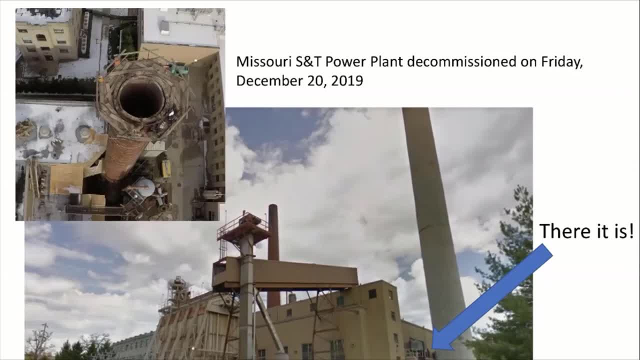 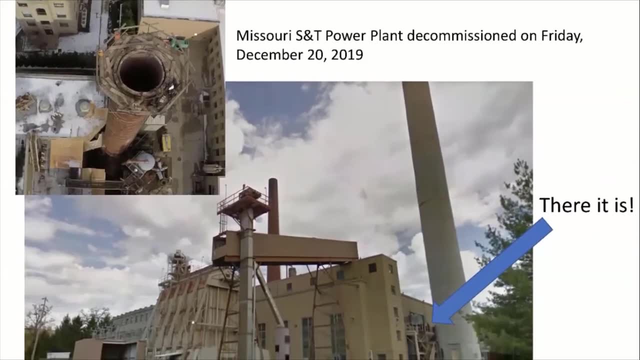 we should put or how we should control the PM coming out of the fossil combustion. But I did manage to take a few pictures of the of the power plant, so I didn't take this one. I guess this is going to be quite dangerous to take. 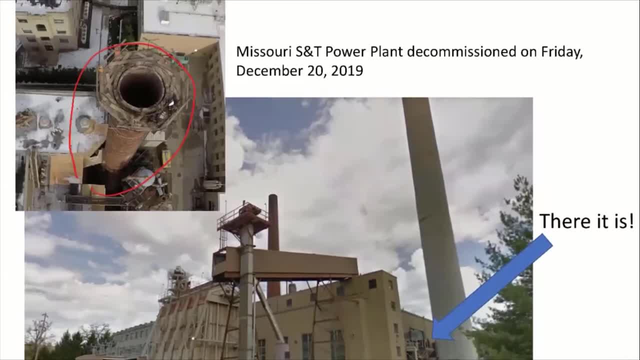 but you see that actually last December we started to dismantle the high stack which used to be a landmark in Walla right. So this is a picture of the high stack which used to be a landmark in Walla right. So this is a picture of the high stack which used to be a landmark in Walla right. 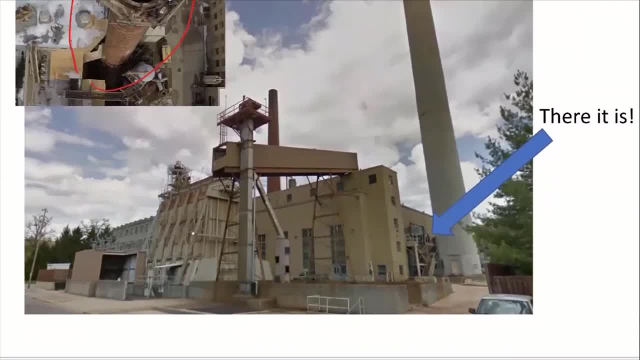 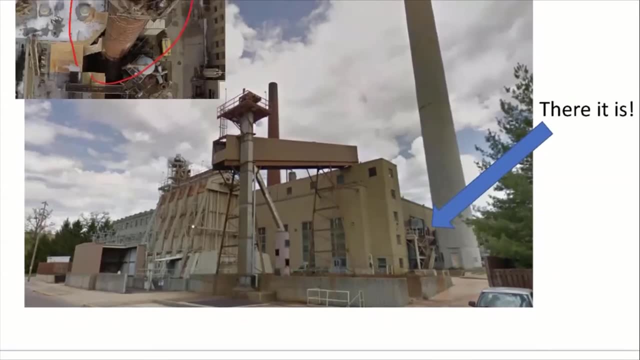 So I'm not sure about the remaining parts, but maybe they managed to leave a few parts still at the original site, but at that time. so I took this picture at that time. the cyclone is located on the side of it. it's here, okay. So you see that it's. 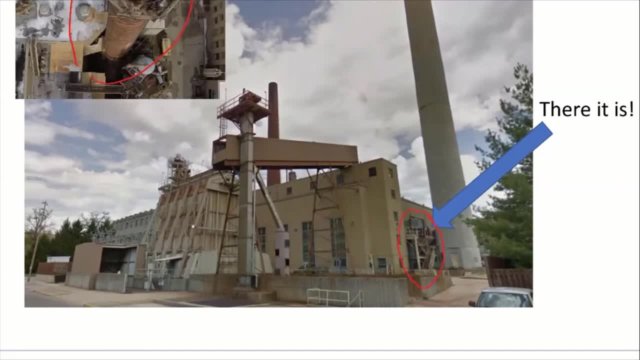 right before the stack. I think there are further PM control devices after the cyclone, because later you'll find cyclone is still not as efficient as other compared to other PM control devices. But this is a direct way you can process the particles coming out of the combustion chamber and then remove the particles. Okay. 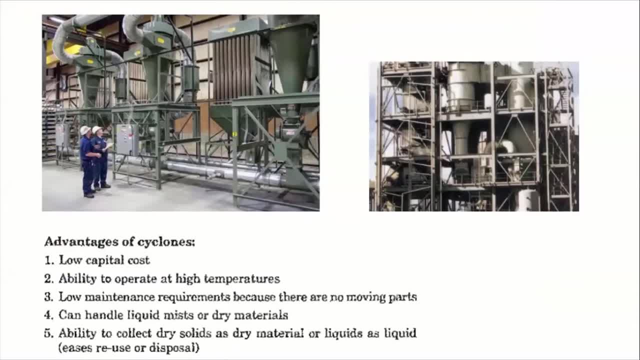 So here are a few other pictures of the cyclones. Cyclones can be large, can be small. you can design different dimensions of it, right? So if you, if there's a large scale coal-fired power plant with a really high- you know- power plant, you can design a lot of different dimensions of it, right? So if you, if there's a large scale coal-fired power plant with a really high, 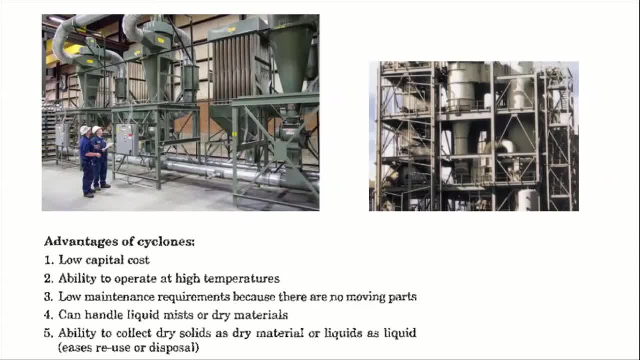 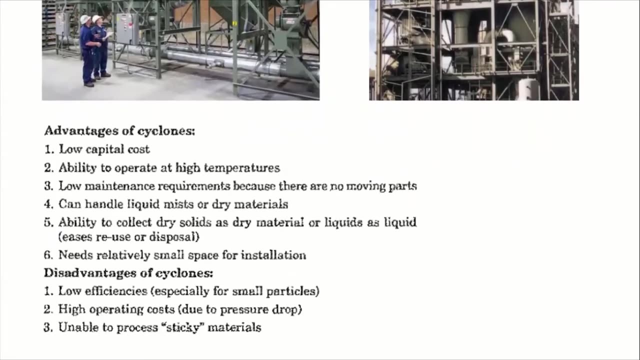 power or capacity, then we can build more cyclones or build larger cyclones to remove the particles. So there are a few advantages and disadvantages of the cyclones, and it's actually quite straightforward to understand these right. So if you think about the, the structure of the cyclone, it's just 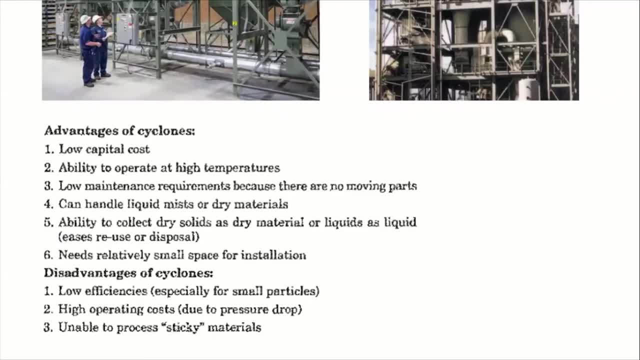 composed of a case, right, a stainless steel or metal case. we don't need to add in any other rotational parts, right? We can just build it as is And we just need to worry about the leakage. There's no leak for the setup right. 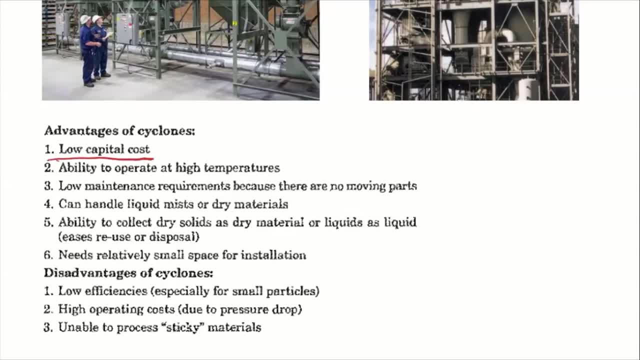 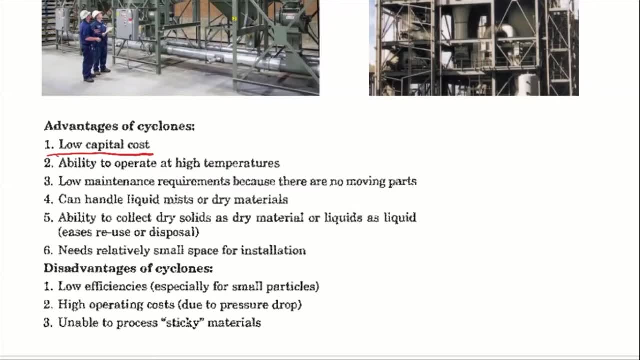 So that's why it has very low capital cost. So I mean we can even build a homemade cyclone, right so it can Operate at high temperatures because the case it's made of metal, so we can withstand high temperatures. It has low maintenance because there's no moving parts. We don't need to disassemble that, you replace. 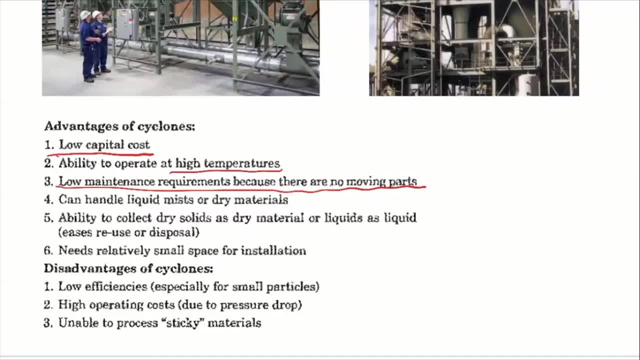 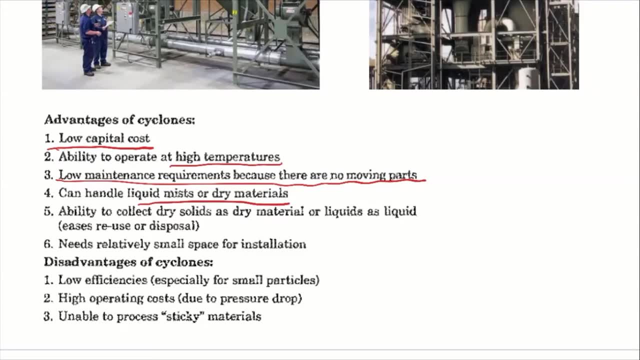 Parts inside because basically there's no parts inside. It can handle liquid, mist or dry materials. Later we'll know that for some PM control devices It cannot control high relative relative humidity particles because it can just block the Device right. it can collect dry aerosols or dry solids or liquid. 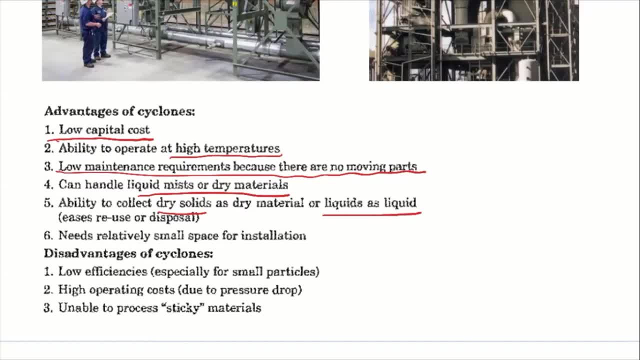 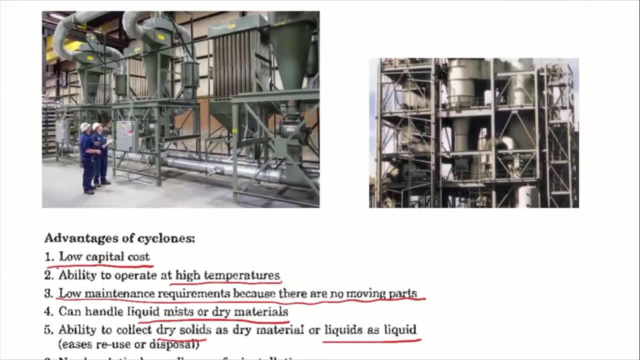 materials. either way works Right. and also it needs, that is, more space for installation. This is mainly because the air flow going through the device has a very high speed Right. to maintain that high speed, the device have to be small. If the device is too large then it's going to create a high pressure drop. 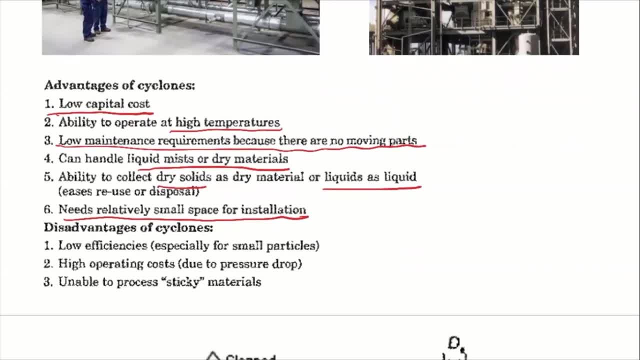 So there are also a few disadvantages of the cyclones. So, for example, the most important one is that it has low efficiency for very small particles. So there are some values in terms of the future or in terms of the removal efficiency, So in terms of the overall PM. 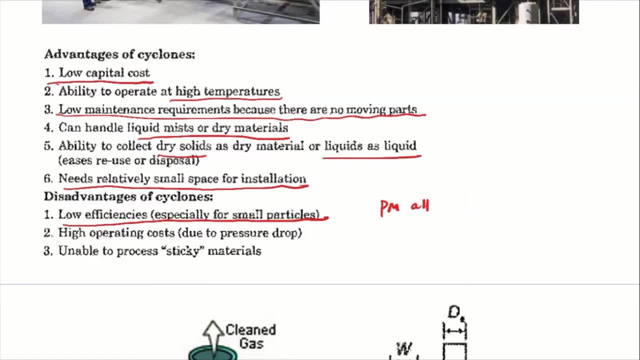 Efficiency This way. so in terms of all the particular matter, We know that there are very large particles. large particles, They have heavier mass so they can get easily removed by the cycle. So in terms of the overall PM removal efficiency That's somewhere around 70 to 90 percent. 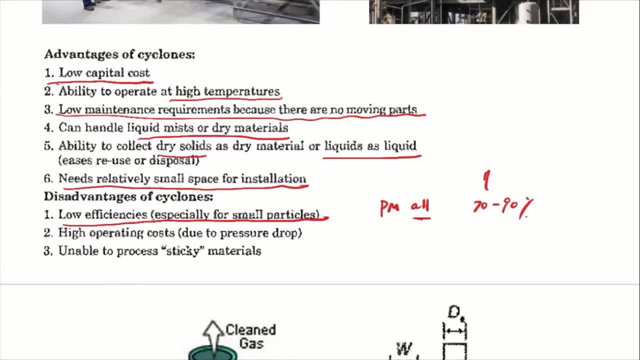 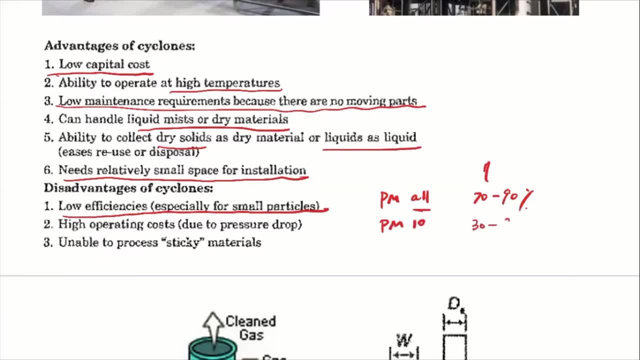 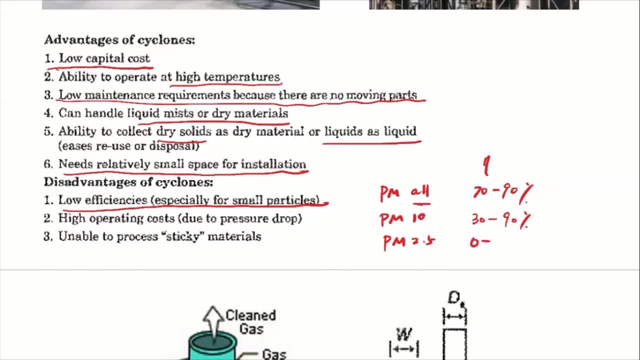 Which is not bad. right, so we can get rid of most of the particles. but if we further zoom in to PM 10, Then that efficiency is 30 to 90 percent, depends on structure. If we talk about further, smaller particles, That's just 0 to 40 percent PM 2.5. 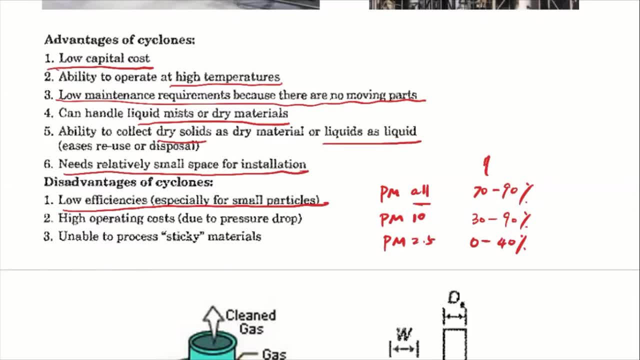 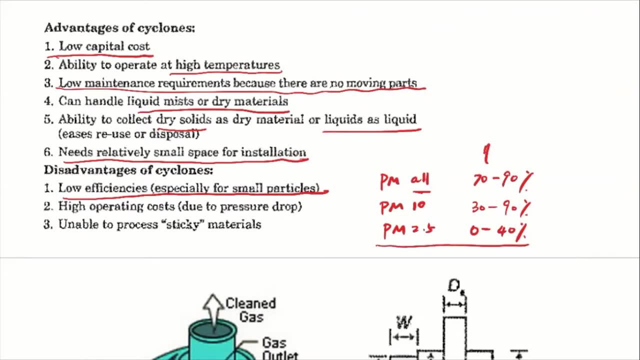 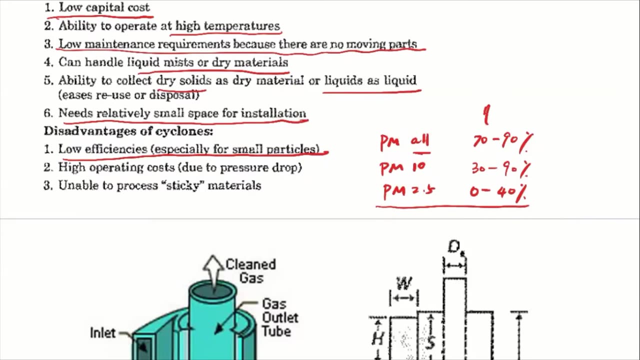 So the the cycle doesn't work very well. So under this situation we have you, You, some other devices to remove very small particles. so Here you can also see that how people will show the overall efficiency. So a lot of coal-fired power plants- when I talk about their PM, remove efficiency. 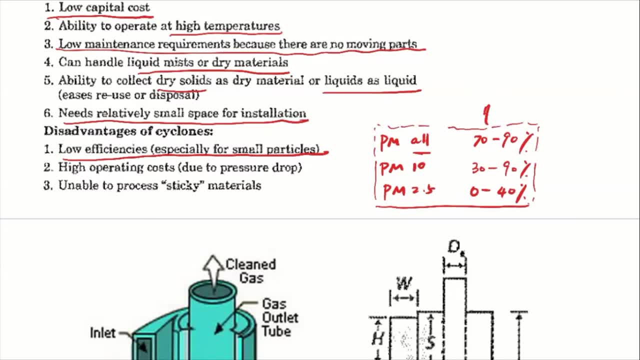 They will say that the removal efficiency is 99.9 percent, But that is the overall efficiency, right? So in terms of the very small particles, the efficiency can be very low. And these small particles because they can suspend in the air for a longer time, so they can put a more health. 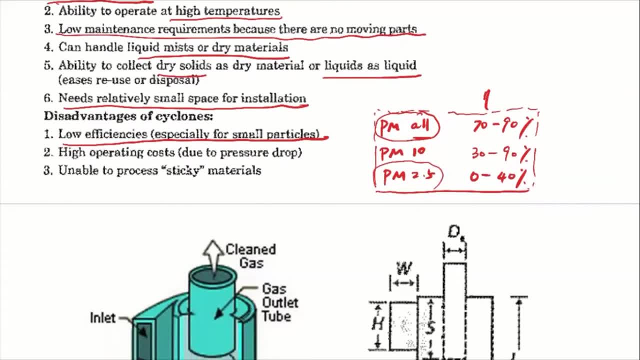 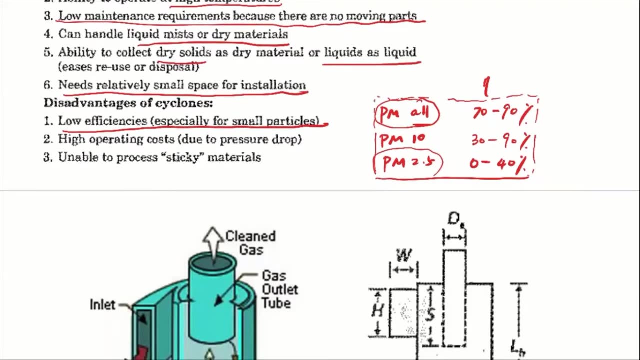 damage to human. So you can. from those words, you can basically understand: People try to bring up their highest efficiency, but in details it might not look very good. Okay, So the other advantage is that it has a high operating cost because of the pressure drop, because 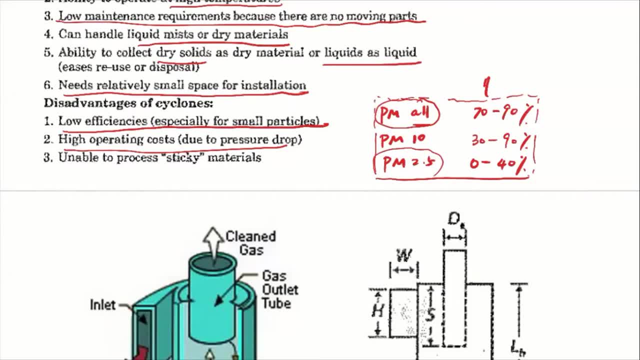 We have to pull the air flow through the cycle, So that's why we have to put a fan downstream of the cycle to draw the air going through right and sometimes, So, basically, because of the centrifugal force. the higher efficiency we want, then, the higher the speed the particle should be. 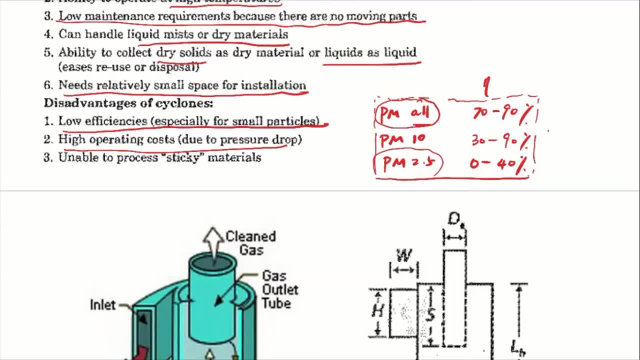 right because, again, the centrifugal force is Mv squared divided by R right. So if the velocity is becomes higher, Then the centrifugal force will become, or the required centrifugal force will become higher, which means that smaller particles cannot sustain them in the rotational. 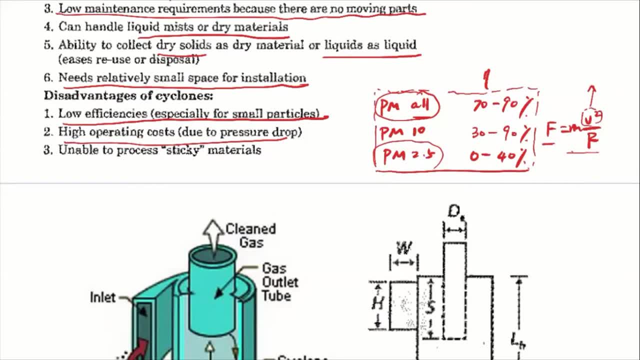 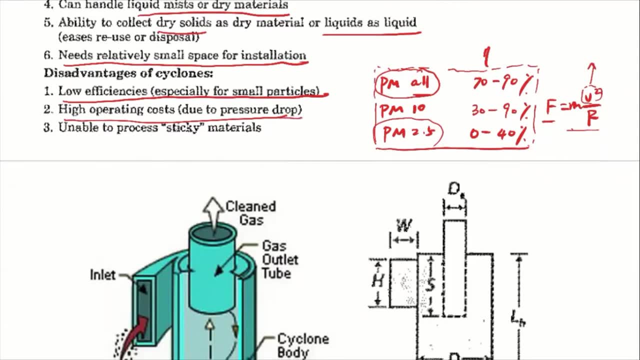 So that's why we have to bump up the speed. But once we bump up the speed, then the pressure drop will become become higher, right, so it's going to take a Cost more in terms of managing or maintaining this device. the third of disadvantage is that 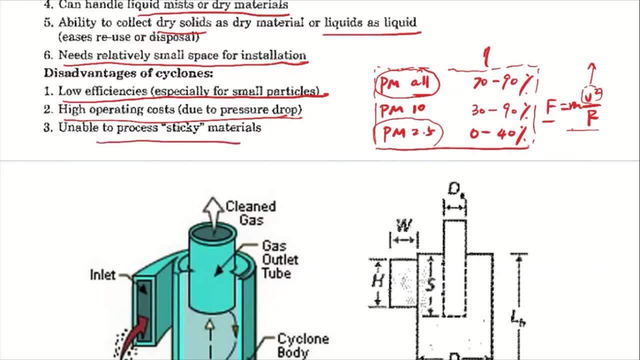 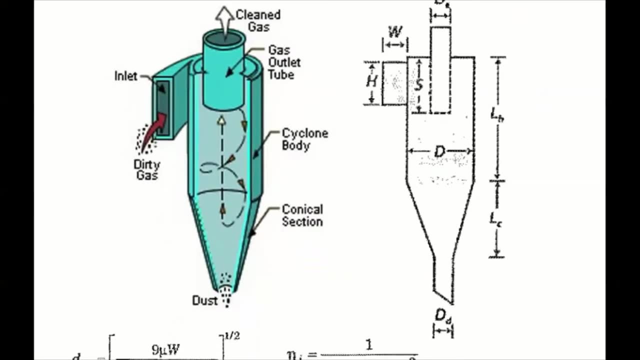 it's unable to Process its sticky materials. So it's also quite straightforward: if particles is very sticky, It's just going to stay on the wall. There's no way we can collect them at the bottom. So here I'm showing a few Schematic diagrams of the 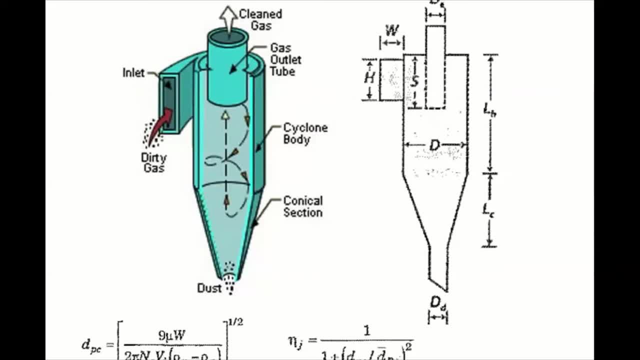 Cyclone and see that the internal structure is also quite simple. So basically the air is introduced from the side of the cyclones right, and then after it enters, It's going to have that rotational movement. So I also mentioned that, for example, in that Homemade cyclone you can see that the air actually moves. 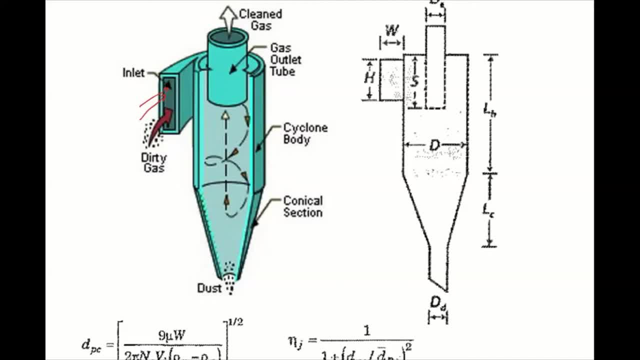 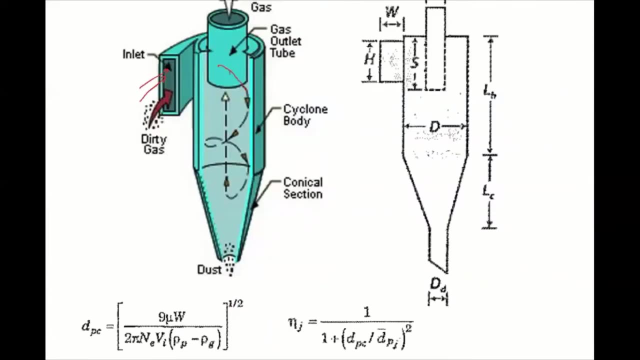 Similar to a ribbon right, So it's not going to compress or basically stack on each other, But they have to align very well, because the air is not compressible in here. So that's why when the air first come in, it's going to rotate and then it has to go. 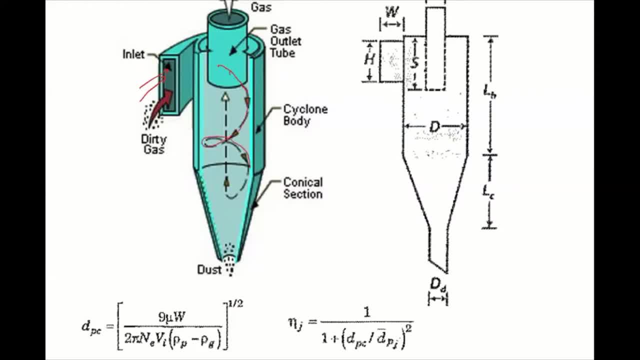 Further below right in this way and then further Go below here, So at the bottom, because of the conical shape, so there's no more space for the air to further move down Right, and then at this time the air will just come up, mainly because the outlet is here. 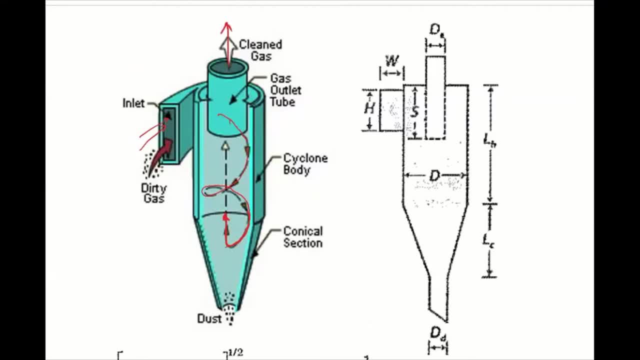 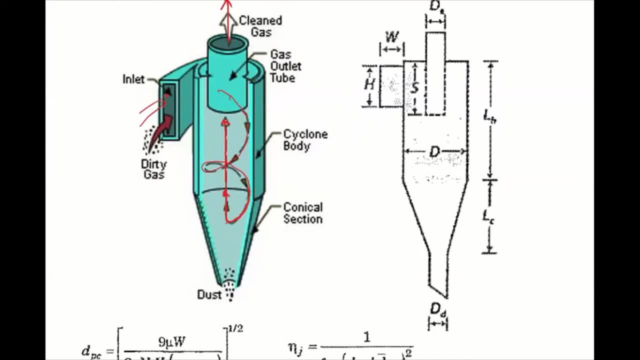 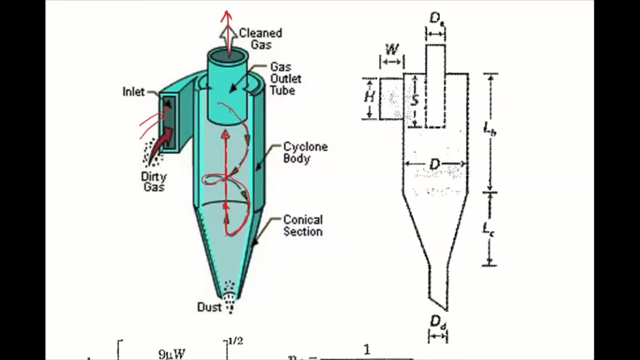 Right now that continuously draws the air from here, right? So the air will finally come up. so in terms of the efficiency of the cyclone, So you can see that basically the efficiency would be determined by how many turns Makes in the cyclone, right? So if we make a very long 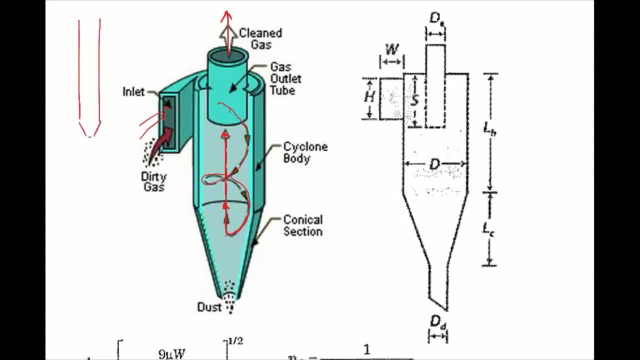 Cyclone have a very long cylindrical shape, then it can make more turns Right before it's introduced outside, before it's emitted outside right. So the more these turns it can make in the cyclone, the higher the efficiency and actually the number of turns is. 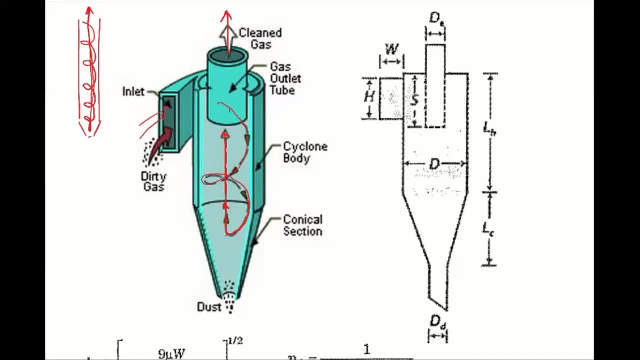 Dependent on just a few parameters, right? So we mentioned that the air will move as a Ribbon, right. So the number of turns would just be dependent on the height of the airflow that's being introduced, Right, and also what is the height for the entire cycle. 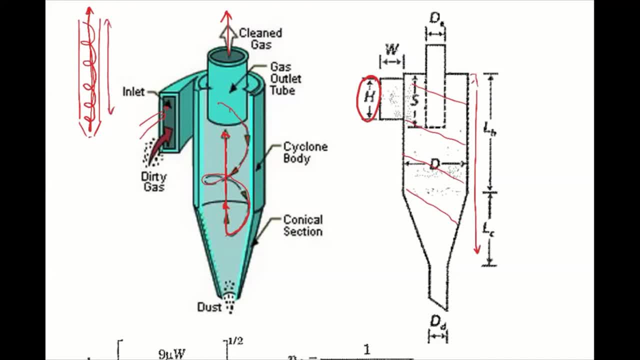 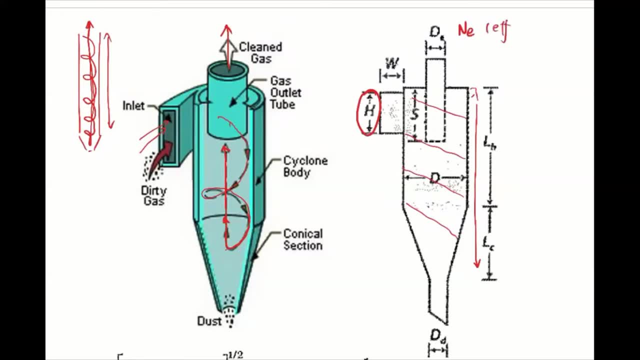 Because the longer the height, the more turns they can make, Right? So we call this turn, we use the parameter called NE. This is the effective turns. So the effective turns can just be calculated by LB plus half of the LC divided by H. okay, so LB is. 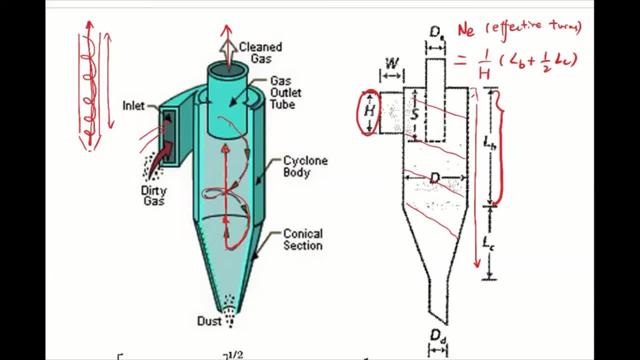 The cylindrical part. Okay, LC is the conical part. It's the height of the conical part. So we can just use this height and then divide by the height of the inlet flow to calculate how many turns, or how many effective turns, the air can make in this cyclone. 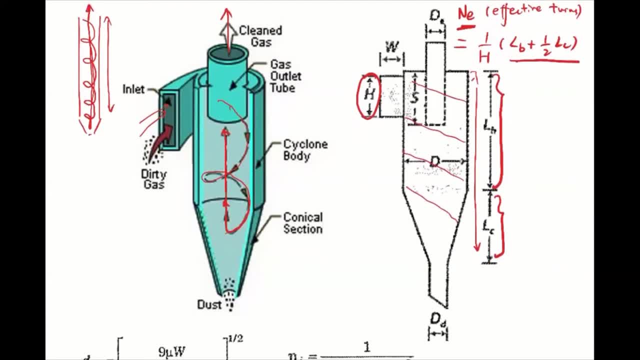 And then the other thing that will affect the collection efficiency is the velocity, the air velocity. We know that the air will be introduced in this way. So if we look in this angle, the air will go inside. The air will go inside. 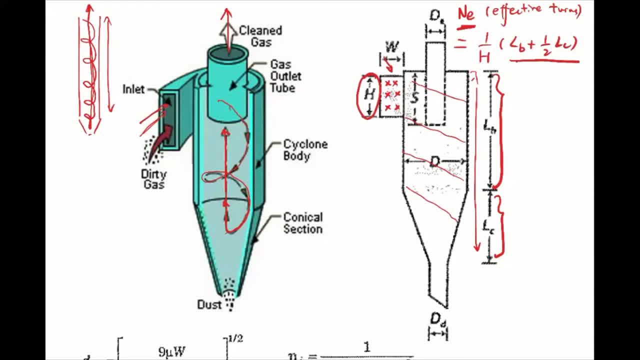 So that's why we can see these crosses, basically the arrow pointing towards the screen, And then the air, after getting inside, is going to rotate in this way. So the velocity of the air will also determine the efficiency. I mentioned that the higher the velocity, the higher the efficiency. 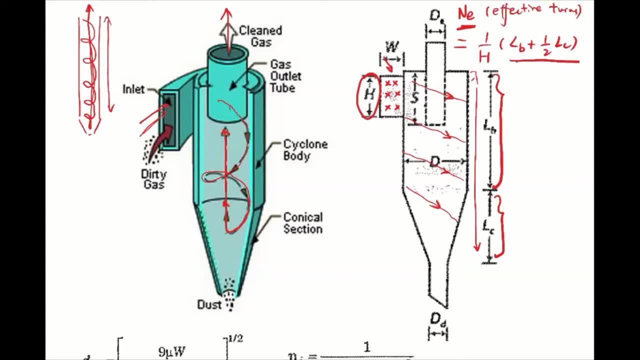 Because the higher the velocity, the higher the centrifugal force. So this velocity- Here people use VI, which basically means the inlet velocity- can be calculated by just the flow rate divided by the cross-section area of the inlet. So it's just Q divided by H multiplied by W. This makes sense. 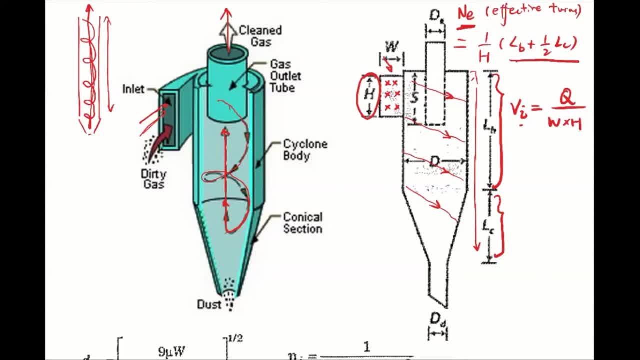 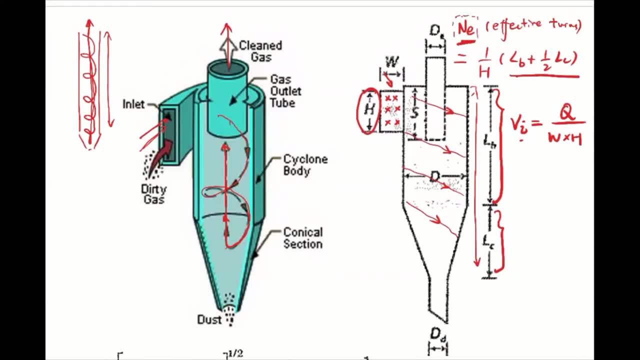 We have the flow rate divided by the cross-section area, That's the velocity, which is the inlet velocity. So basically, with these parameters we can try to solve, for what is the collection efficiency of the cyclone right? So this is the equation that people come up with. 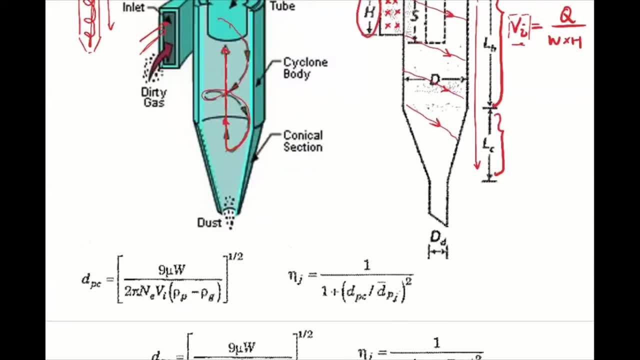 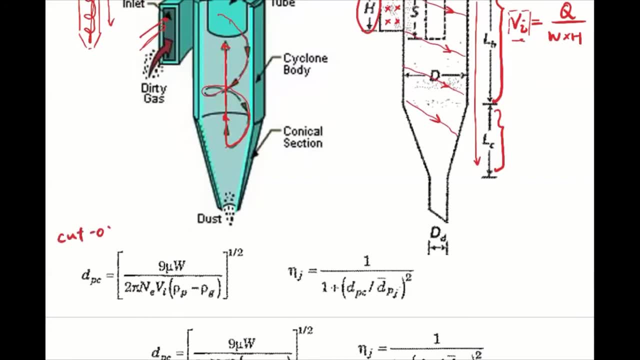 So for each design of the cyclone, people define a parameter that's called the cut-off size. So this is the critical size for a cyclone. So basically, if the particle has a size that's larger than this critical size, it's called six- Hotel 50.. So it's very, very large. So if the particle has a size that's larger than the critical size, the toppiece size V then is the вес of this particle. This will be to friends, And then the efficiencyاص spicy. 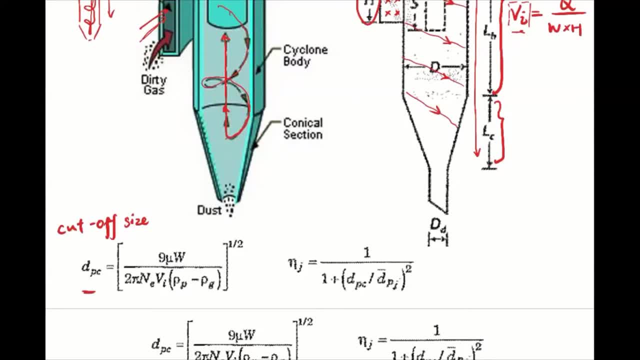 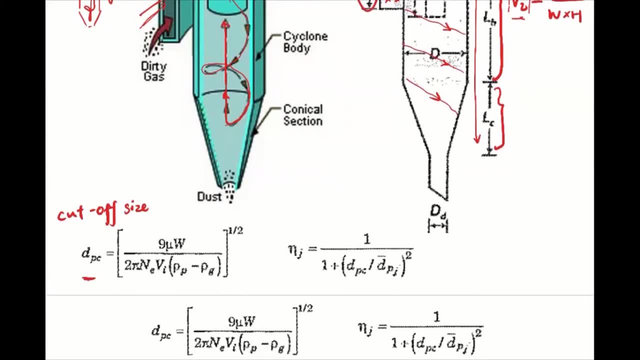 Decreasing microwave, then it's going to have a higher collection efficiency. but if the particle have a smaller size, then the efficiency will become lower. So this critical size is calculated by this equation. So it looks quite complicated, but we'll show what is the reason it has this form, because now we know the 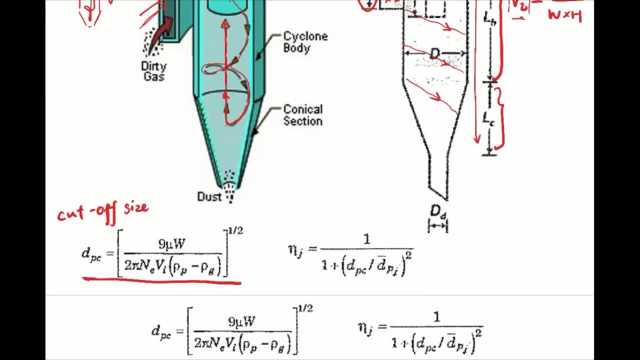 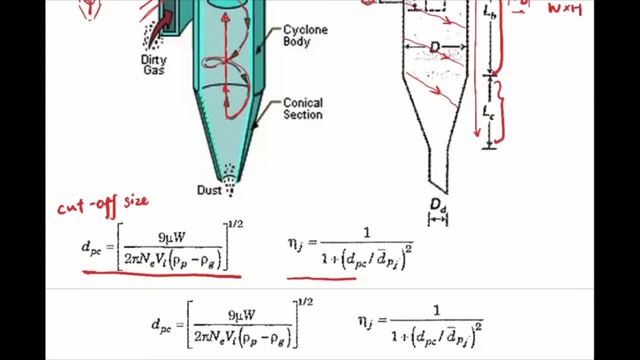 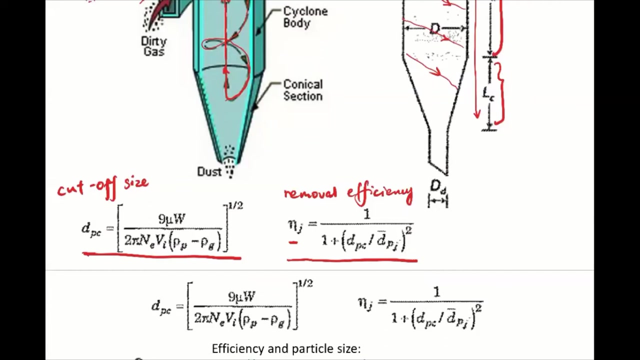 equation for the drag force. This is actually quite straightforward to solve for this equation. So on the right-hand side it's the equation that calculates the removal efficiency, So the eta here. So this is the removal efficiency. So the removal efficiency is specific for particle with the size of the. 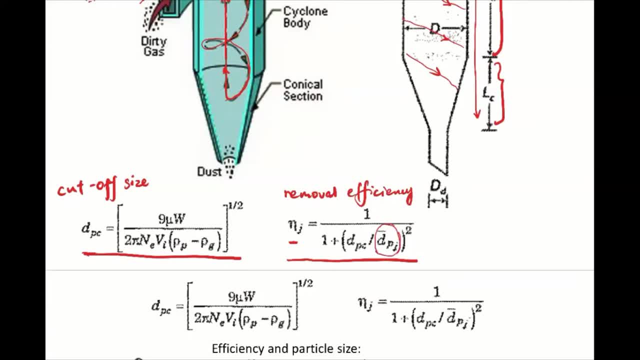 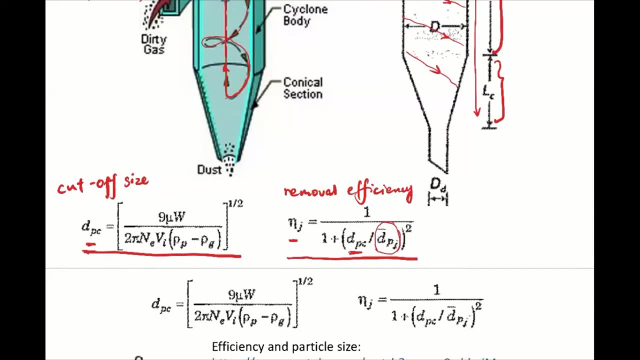 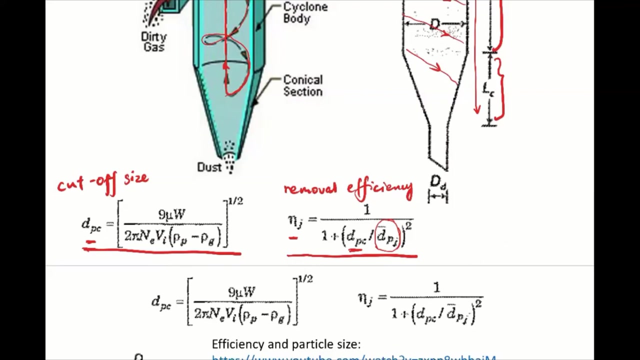 dpj. Okay, so I already solved the dpc here. You see, the dpc is just the equation here. Maybe I should leave some time for you guys to write down the equation. Okay, so this is the cutoff size: dpc. So for each, basically for each of the 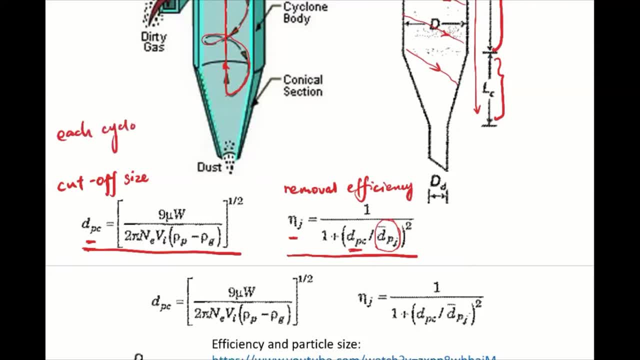 cyclone. this is the cutoff size dpc. So for each, basically for each of the cyclone, it's going to have a specific cutoff size. So we have to put in the parameters So you can see that the parameter is dependent on the W, which is the width of. 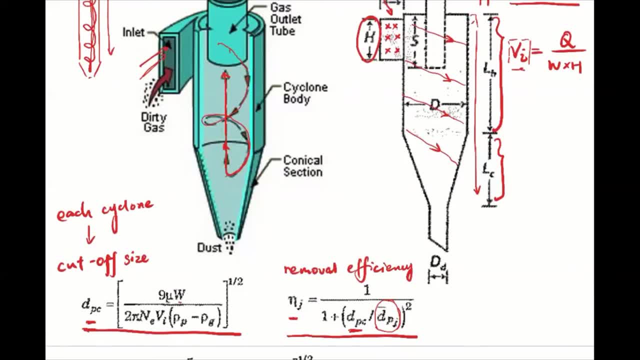 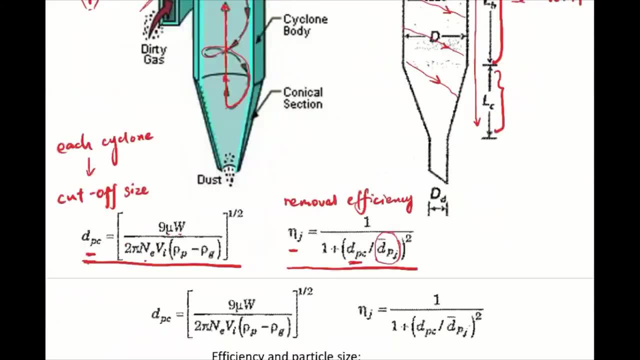 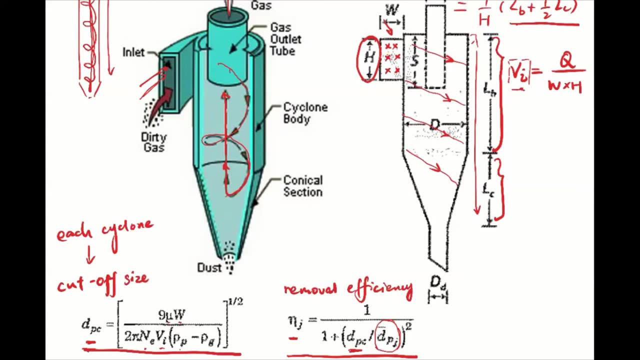 the inlet right, Mu is the viscosity of the air and E is the number of effective turns we just introduced here. Vi is the inlet velocity, rho p is the particle density and rho g is the air density. Okay, so with these parameters we can solve for what is the cutoff size right? 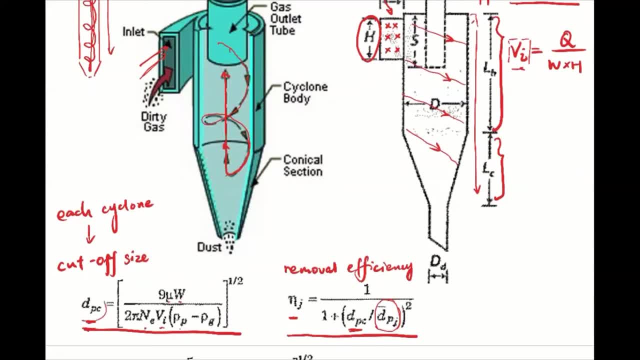 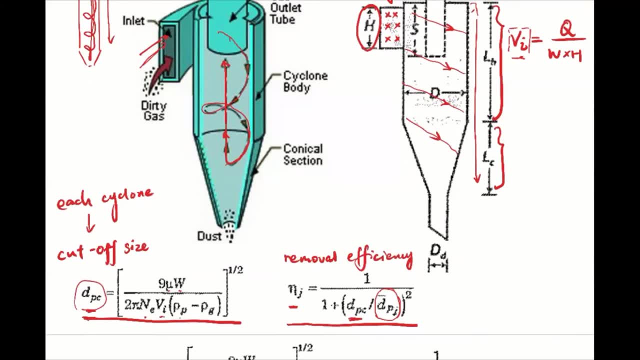 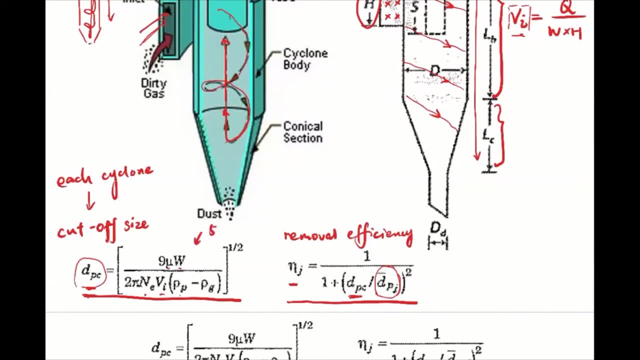 And the second equation here basically use this cutoff size. So if we know particles of a specific size, then we can calculate what is the removal efficiency. okay, So let's say, for example, for a cyclone, we find out that this cutoff size is 5 microns. 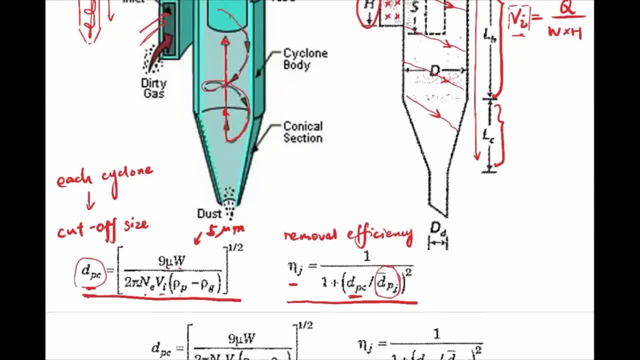 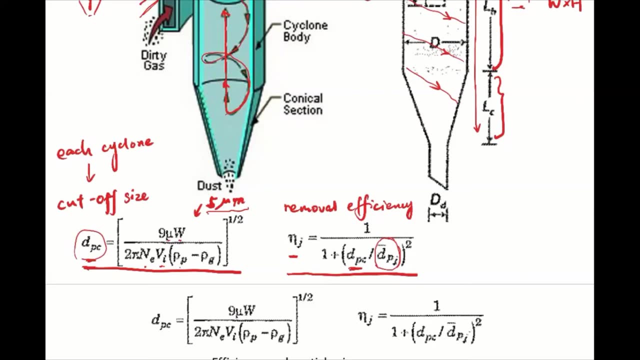 Basically, we'll plug in some numbers later on. Let's say for a cyclone, for example, cyclone. After we plug in numbers, we find that this size is 5 microns. What we're going to do is to plug in this 5 micron to here. 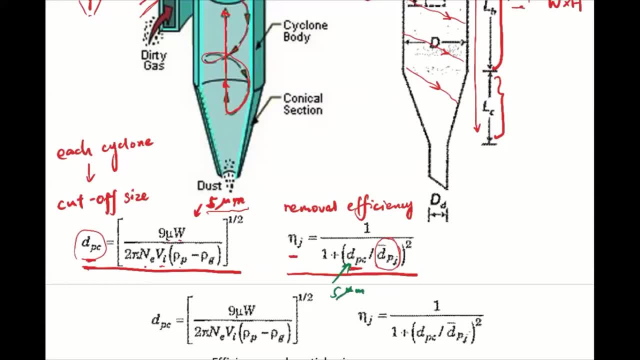 Here we'll put in 5 microns And then for this size it's any size that we're interested in. So, for example, if we're interested in the collection efficiency of 5 micron particles, okay, so we introduce 5 micron particles into. 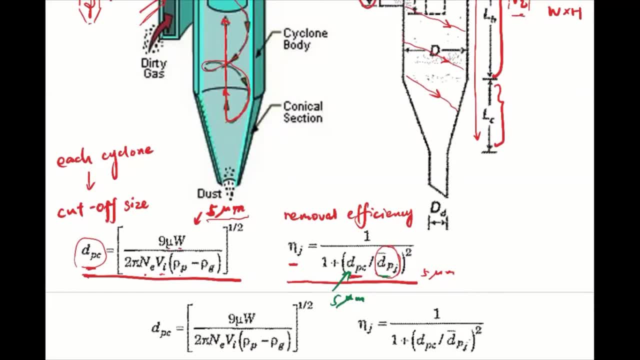 this cyclone and then operate it. So what's going to be its final efficiency? E to the 5 micron is going to be equal to 1 divided by 1 plus 5 divided by 5 squared. okay, That's 50%. You can see that the cutoff 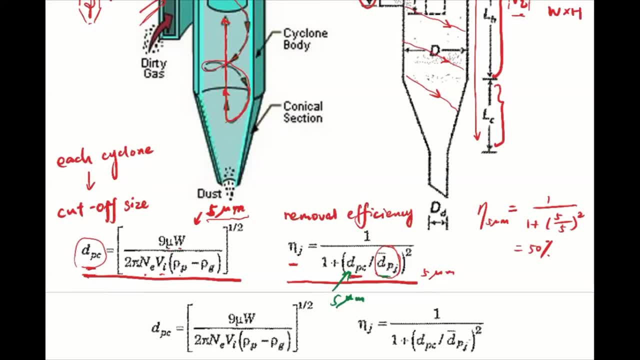 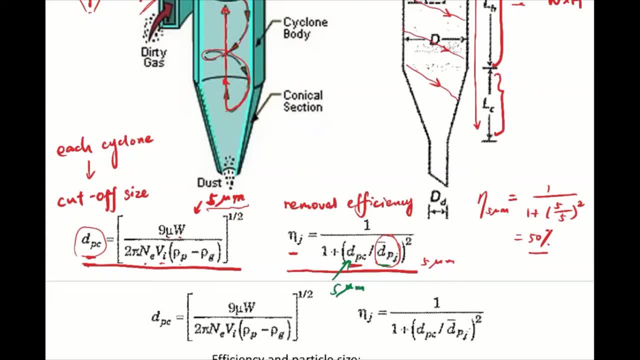 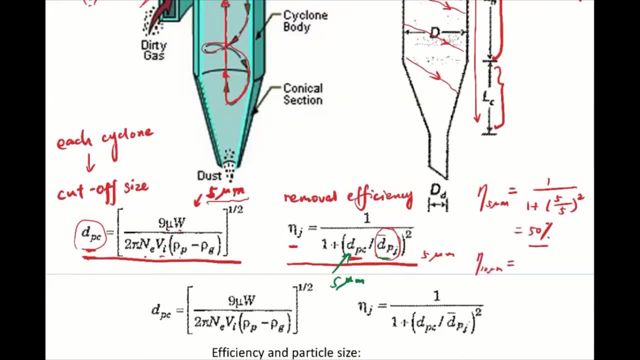 removal efficiency, right. So now let's say that we're interested in 10 micron particles. So E to the 10 micron is going to be equal to 1 divided by 1 plus 5 divided by 10, okay, squared. So that's 1 divided by 1 plus this is 0.5, right. 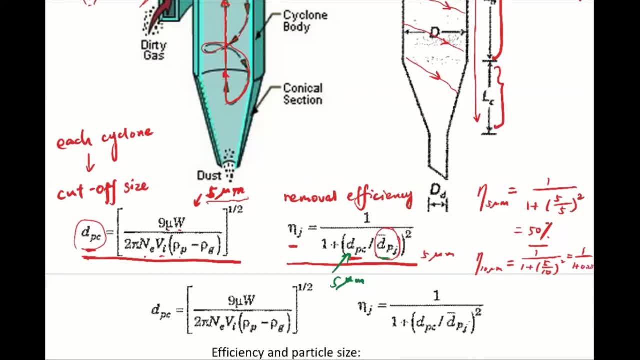 So 0.5 squared, that's 0.25.. 1 divided by 1 is 0.25, right? So that's going to be 80%. So you see that from this equation we can get a general trend. Let's say: 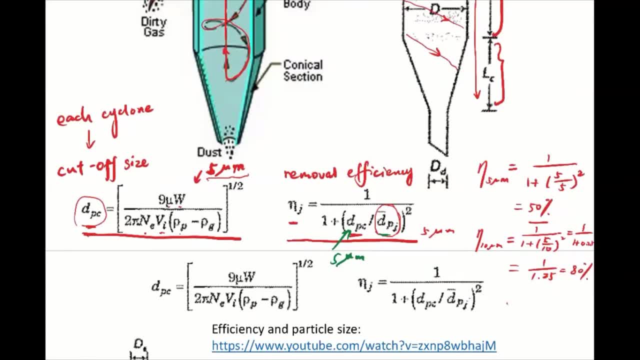 that what's going to happen if particle size increase? If it increases it, efficiency is also going to increase, right? So let's say, for an extreme example, right so we talk about particles of a few microns. Let's say we use our 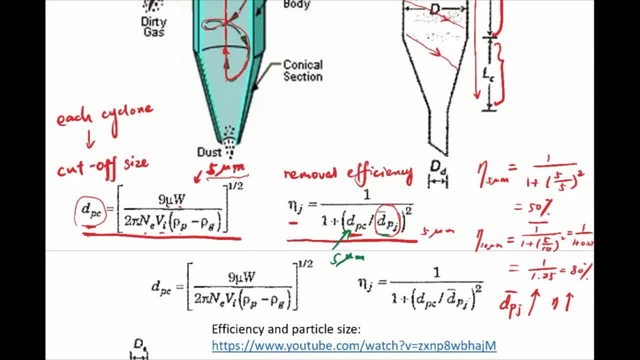 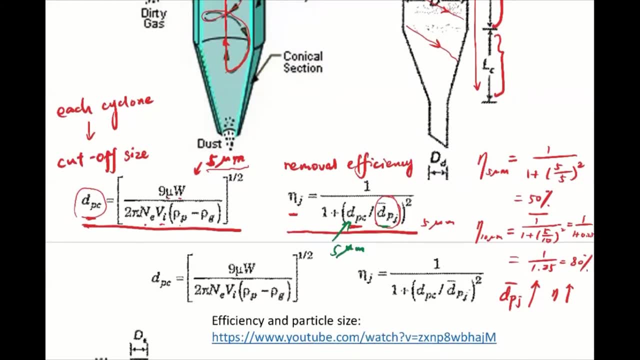 classical example of a particle use: a potato. okay, Let's say we put a potato inside because the size is too large compared to the critical size, So this term will go to almost zero, right? Five microns divided by a size of a potato, and then 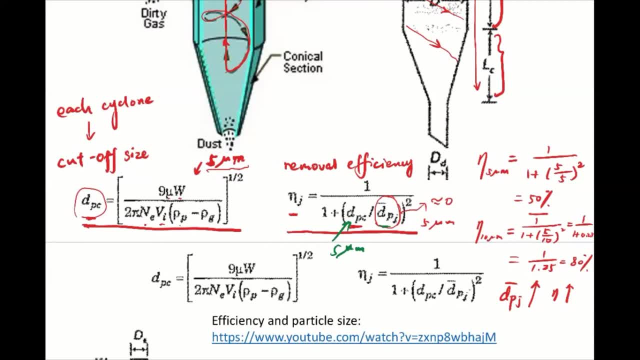 further square it, So this term will go to almost zero. So that's just 1 divided by 1, which is 100%. okay, If the size it goes to extremely large range, then the efficiency is 100%. But what happens if we talk about very small? 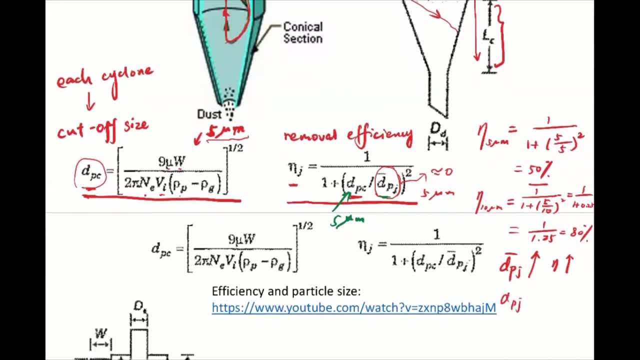 particles right, TPJ decrease. let's say, if the particle is very small. We're talking about one nanometer particle, or even air molecule. Air molecule's a few, maybe a few tens of, maybe point something: nanometer, 0.1 nanometer. let's say Then. 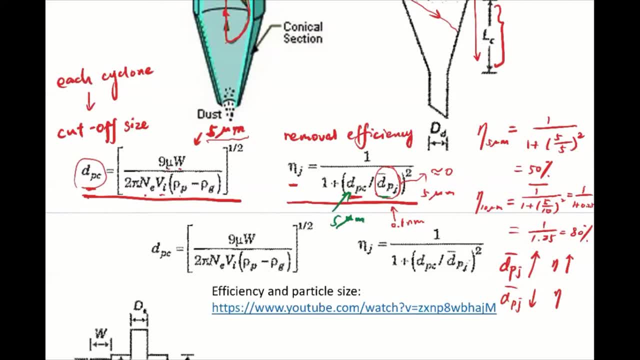 DPC divided by DPG will be very large right, And then you further square, it will become more, basically, much larger, okay, Infinitely large. So one divided by an infinitely large number will go to zero, which means that for small particles, the collection. 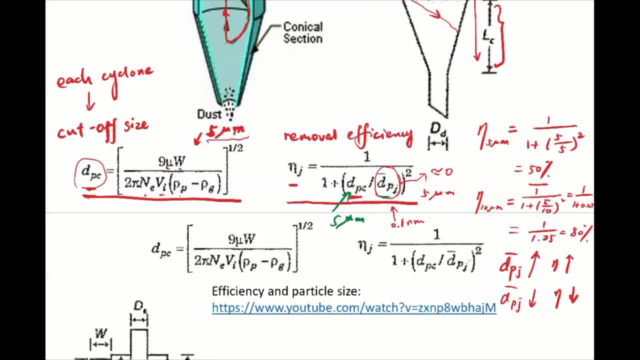 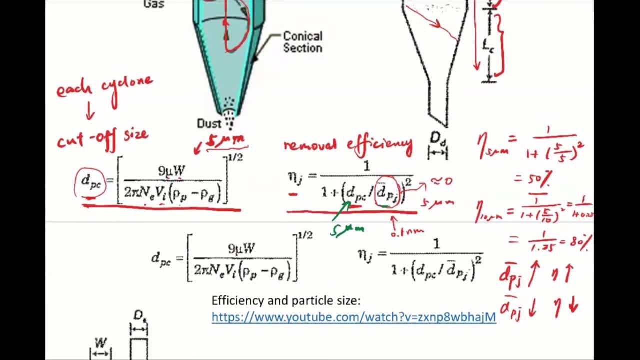 efficiency will be very low. okay, so now you can see how this equation makes sense. so, basically, first to basically, to decide a future, decide a collection efficiency of a cyclone, we first need to find out what is the cutoff size and then, with that cutoff size, we can calculate whatever. 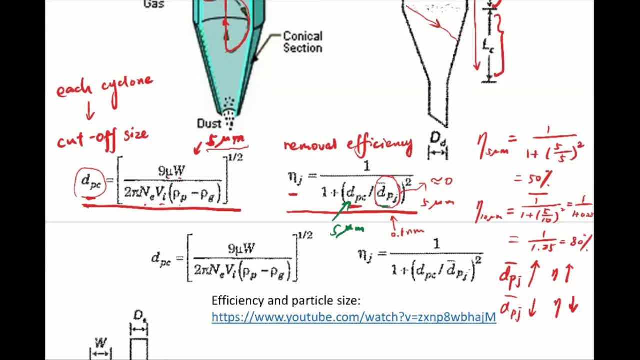 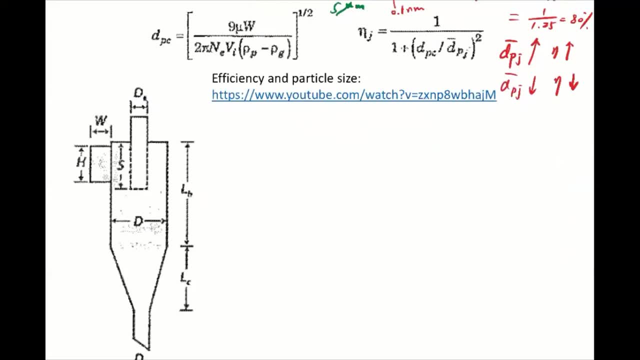 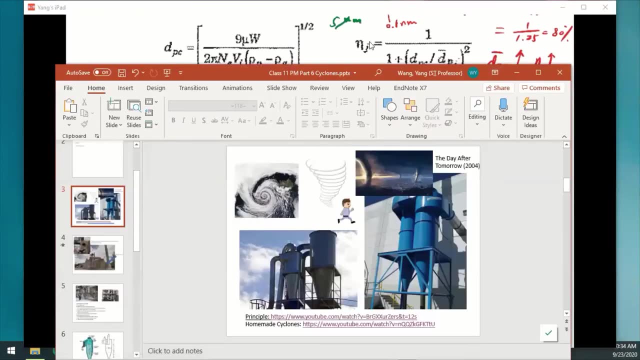 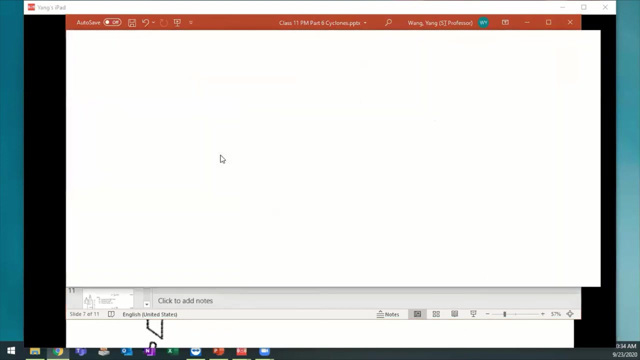 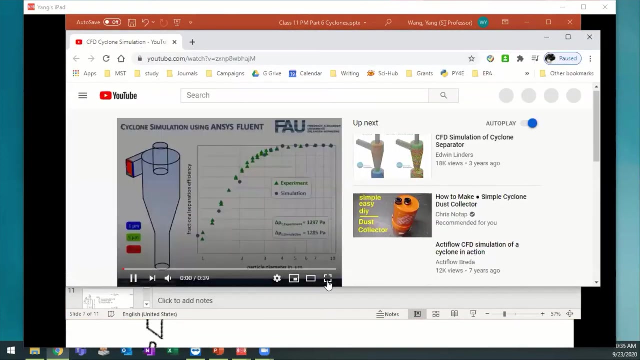 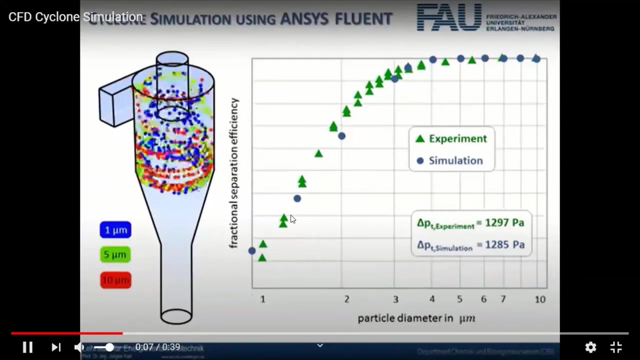 efficiency for a specific particle size, right? so here i have another video trying to show you, basically, particles with different sizes, they're going to have different flexion efficiencies and this is for a cfd simulation result. okay, so you're introducing particles of three different sizes: one micron, five micron and ten. 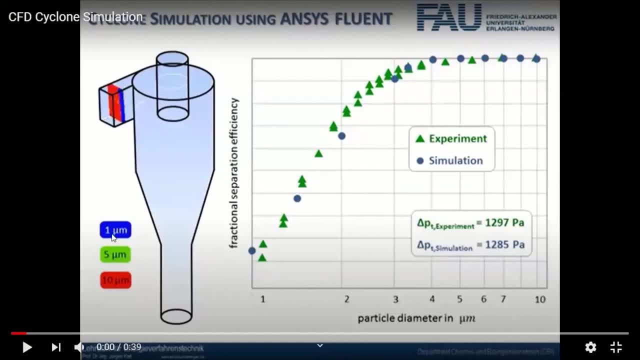 micron. okay, so the one micro ones are just blue ones. so you see, because of their smaller size, the small particles wasn't just follow flow And then they can easily get exit from the settles, While the larger particles they will just stick to the wall and then finally get collected at the bottom right. 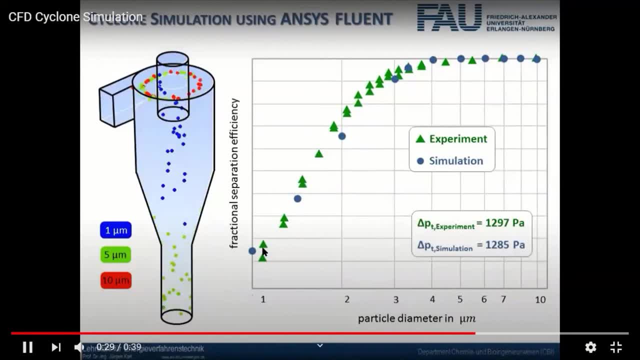 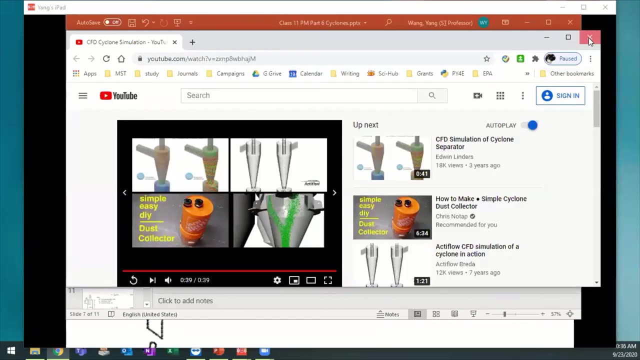 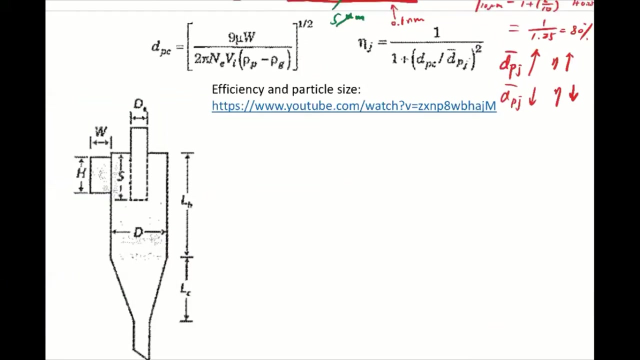 So basically from the simulation you can calculate what is the collection efficiency for particles with different sizes, And then actually it agrees very well with the experiments, right? So basically, particles with different sizes, they're going to have different collection efficiencies. 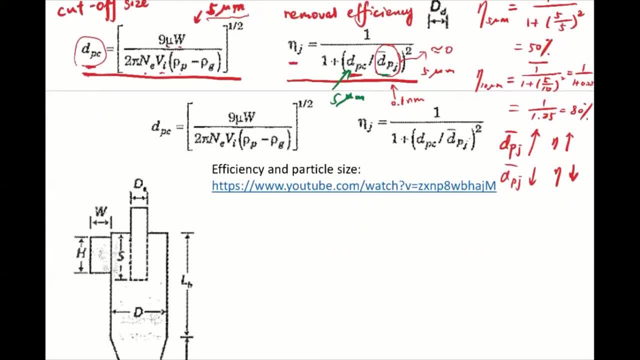 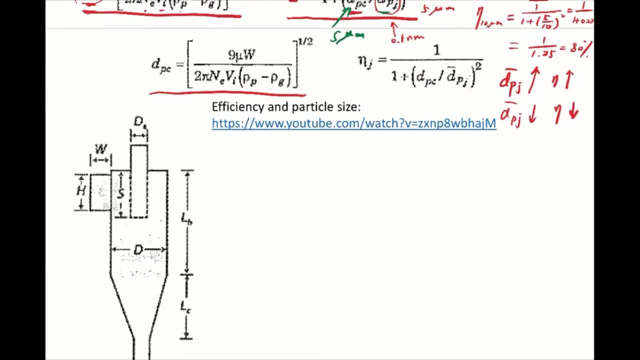 And then, as we mentioned before, for example, this equation, this DPC equation here is very complicated And because now we know the equation for the drag force, we can actually try to Prove why this size is the critical size. OK, 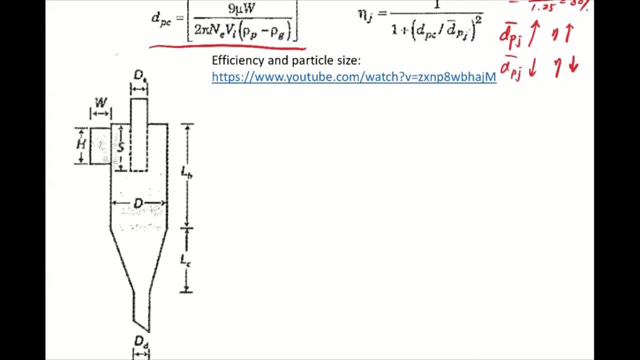 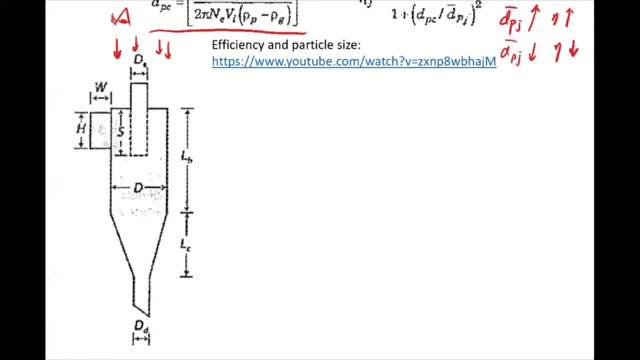 So let's say, for example, if we just draw the cross-section view of this cycle, OK, Let's say we look from the top, right, So what's going to look like from the top is basically a cylinder going to be a sphere. 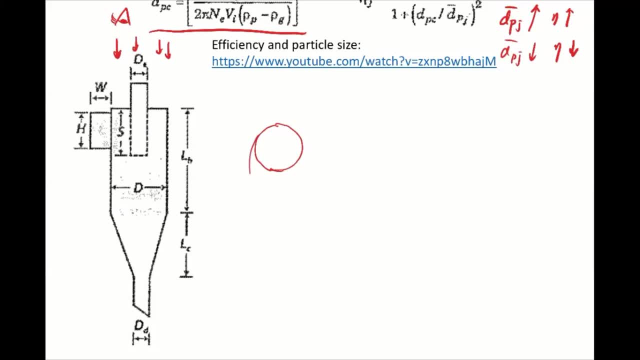 It's going to be a circle, And then this is our air inlet, right? So after the air is introduced, it's going to rotate in this way And finally, this is the outlet of the air, right? So we mentioned that for all the particles that. 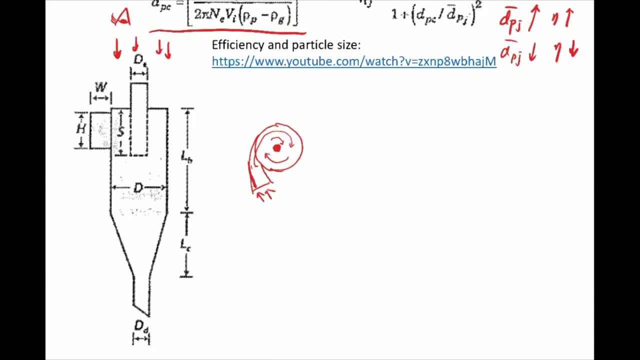 rotates like this, we have to provide a centrifugal force. OK, So it's like we put a string and then connect a string to a sphere and then we spin it. So the force that we pull the string is going to serve as a centrifugal force. 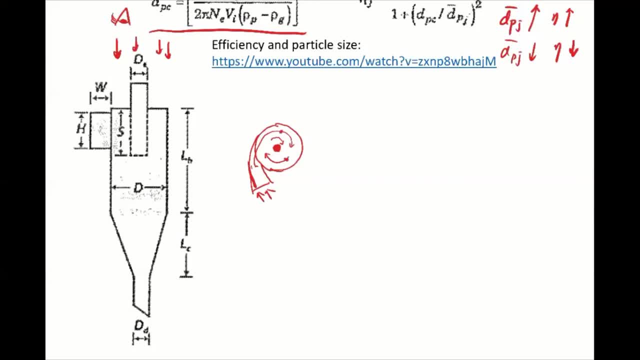 So for a particle to move like this, move in rotational directions, we also need to provide a centrifugal force, right? So where is going to be that force, or what's that force? Because, basically, the air after the particles are introduced in the cyclone there. 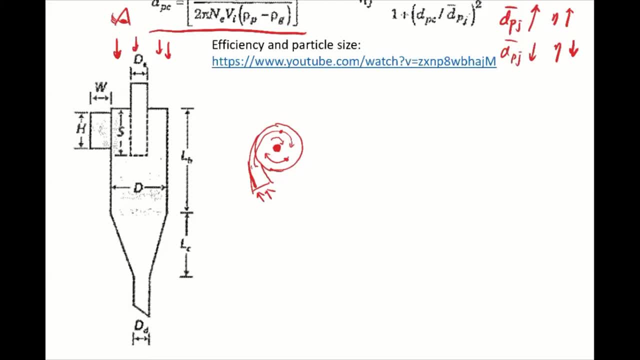 are no more surfaces or no more mechanism to provide this force. right. But one thing we know for sure is that the particles are going to move across the flow, Because, let's say, the particle wants to deposit here, then it has to go across the airflow, move like this: OK. 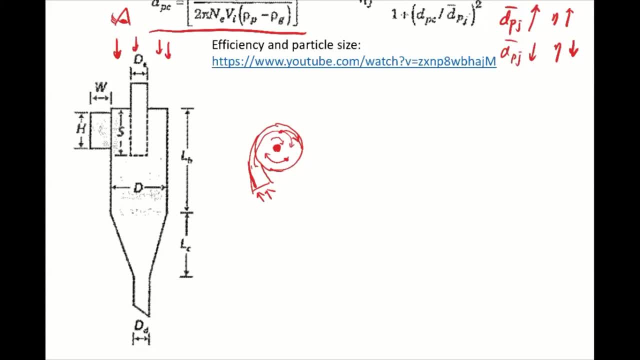 So basically, there is going to be a relative velocity between the particle and the air in this direction right. The particle wants to move from this location to the wall right And then there's going to be a relative velocity between the particle and the airflow. that's. 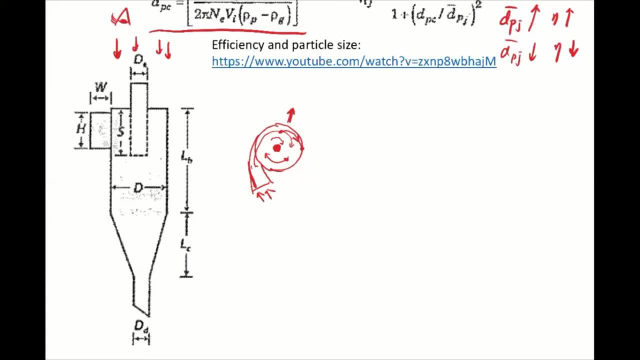 in the radial direction. OK, So once there is a relative velocity, then we know that there is going to be a drag force. So the drag force is going to try to pull the particles towards the center. OK, And this drag force will serve as the centrifugal force. 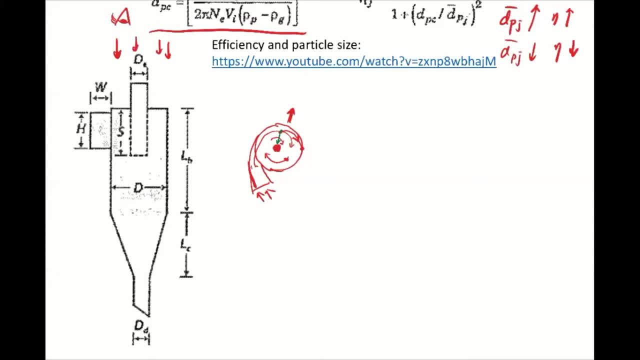 So that's where the centrifugal force come out, right. So basically, what we can do is we can equate this drag force with the centrifugal force. So this is going to correspond to the particle with a critical size, right, It's going to maintain itself. 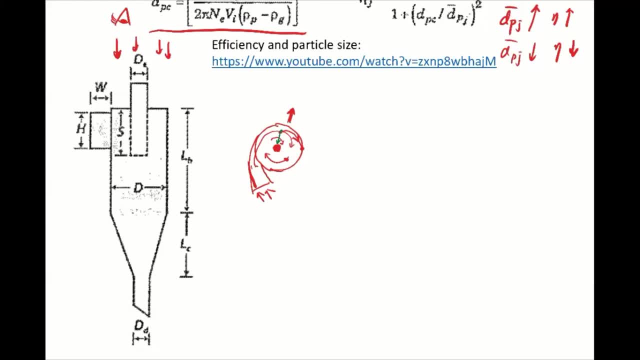 In this rotational flow here. So we know that the centrifugal force is m Vi squared divided by R. So Vi again is the inlet velocity equal to drag force: 3 pi mu dp divided by C, multiplied by Vr right. So this is how we set up the force balance here. 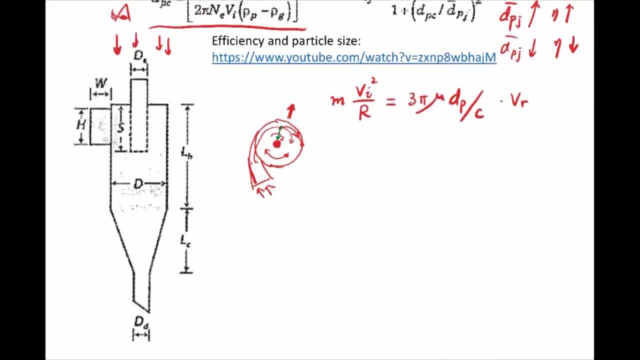 So let's assume that here the particles are very large, So let's ignore this C term. OK, Typically, the cyclones can treat particles of a few microns, So that's why we don't. a few microns is much larger. 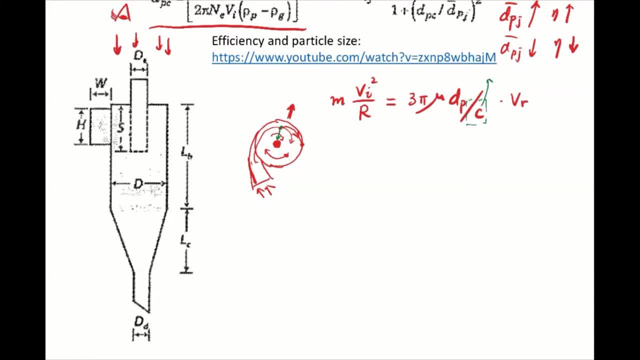 than the mean free path. So we can just treat this Cunningham correction factor to be 1.. So what we can have is just m Vi squared R equal to 3 pi mu dp multiplied by Vr. So again this Vr here, or the relative velocity here. 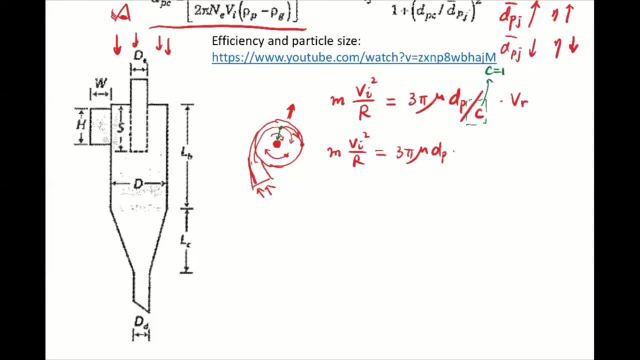 is just the velocity that the particle tries to go across the flow, right, Let's say we set it as Vt. OK. Again, we can put in the expression for m: m is pi over 6 dp to the third multiplied by rho, p, OK. 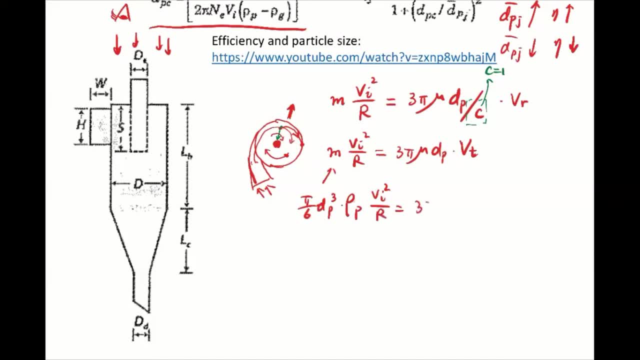 We have Vi squared R equal to 3 pi. mu, dp, Vt. OK, So dp can get canceled. here We have two of the dp's right. So if we just solve with this equation, it's going to have pi and pi can get canceled. 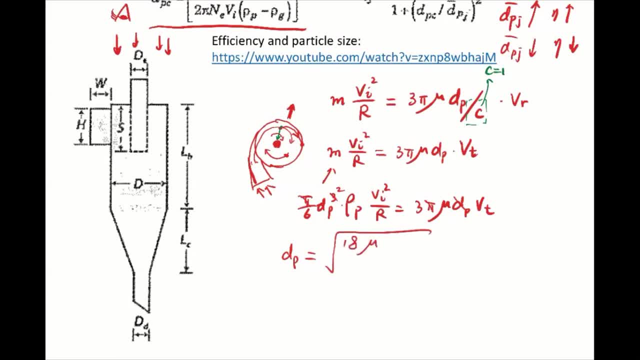 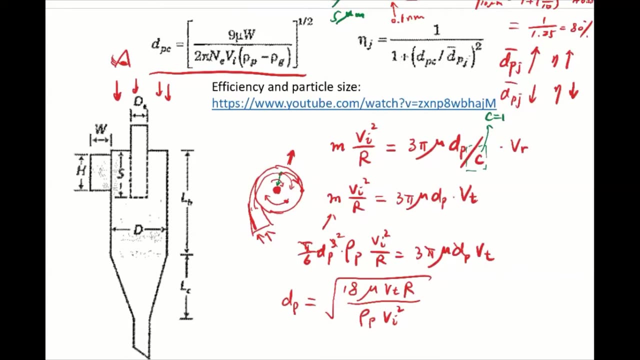 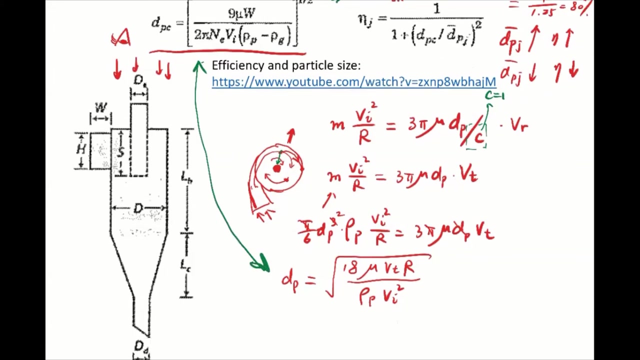 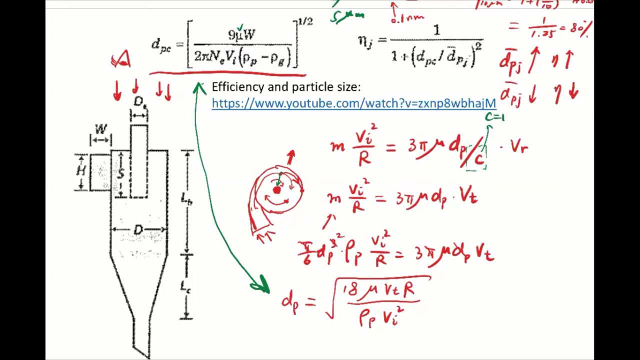 We have 18 mu Vt R divided by rho p, Vi squared, OK. So if you compare these two equations, OK, they are still a little bit different, right? So now we have the mu term here. OK, So we can get. at least we made a, or we. 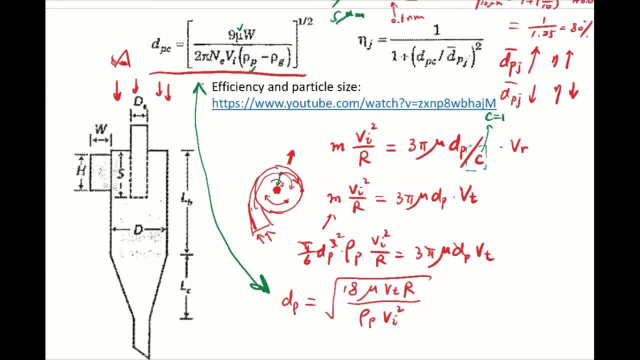 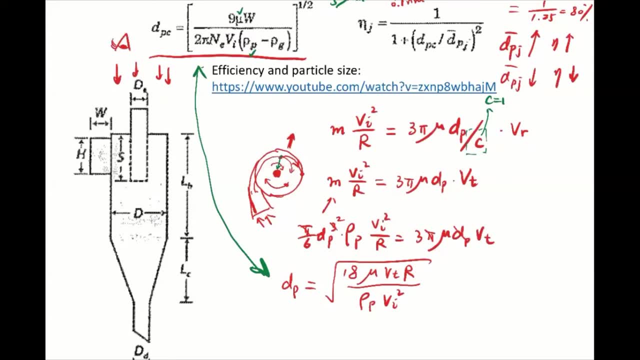 have the particle density term here, So we made some progress here. So the thing is that right now we need to plug in the Vt and Vi, right. So Vt and Vi, Right. So if we add the Vi, it's just the q divided by h multiplied. 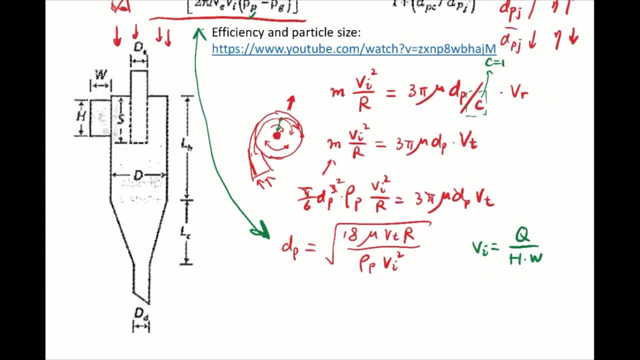 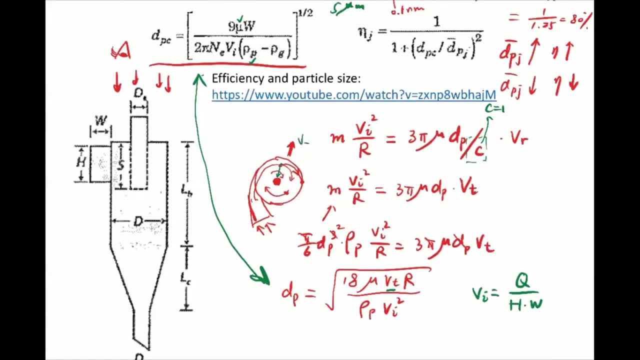 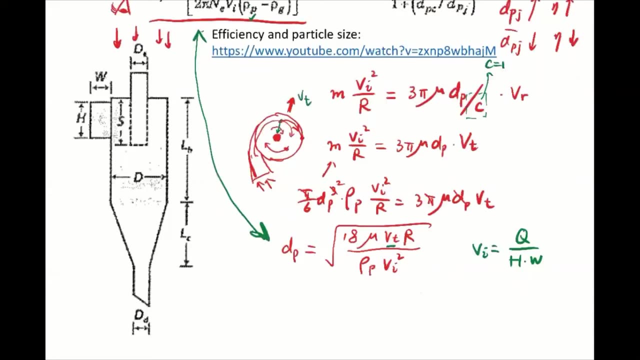 by w. That's the inlet velocity, right. And then we just need to find out what is the Vt. So Vt again is the velocity of the particle that goes in the radial direction, right. So that can be solved in terms of the movement. 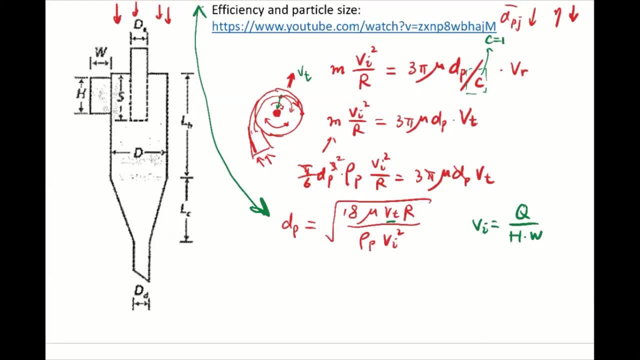 or in terms of the trajectory of the particle. OK, So let's say the particles will spend the time of delta t in this, in this cycle. So one thing we know for sure is that let's say the particles finally get collected, Then Vt multiplied by delta t should be equal to w. 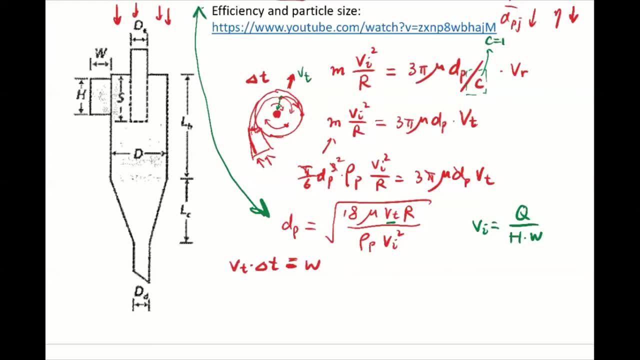 So w is basically this distance here right? This is w Because we know that If the particles can get collected, then it has to enter from here and then spin all the way to the outside right. So this is a radial movement. 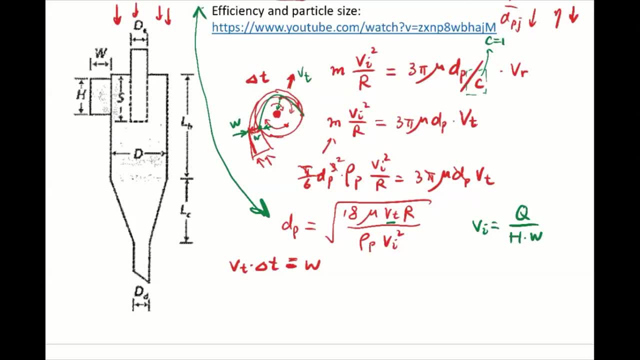 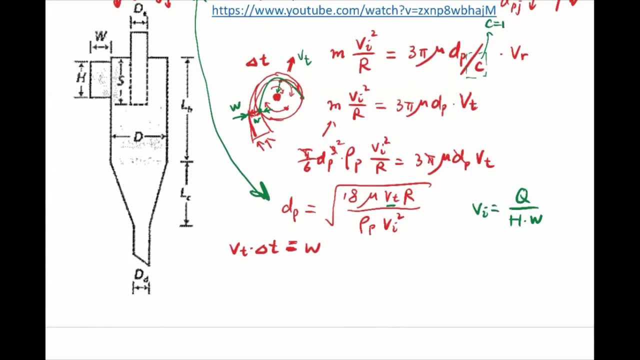 This is a radial movement of the particle, which is w? right. So, at the same time, we know that, in terms of inlet velocity, you know Vi multiplied by delta t, Right, OK, OK. So if we multiply by delta t, that's basically. 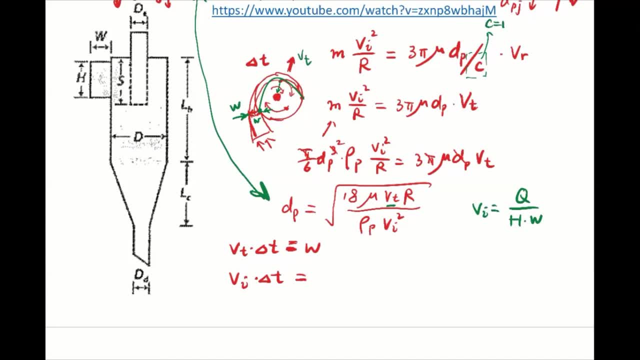 how many turns the particles can make right. So that's going to be Ne multiplied by pi, multiplied by d. So we mentioned that Ne is the effective turns the particles make in the cycle. So Vi multiplied by delta, t, that is the total distance. 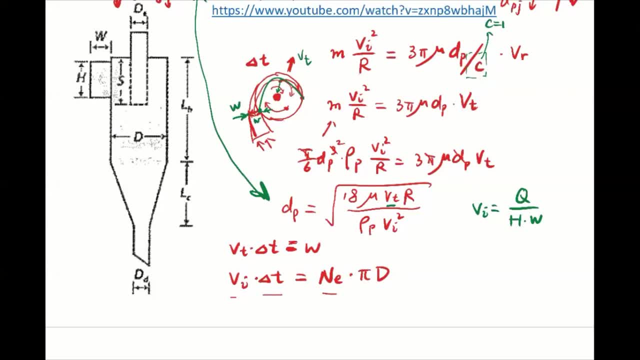 Basically the total distance that a particle make in terms of the rotational movement. OK, So we have these two equations right. So now we know that basically, if we divide Vt, divide these two equations, we can just cancel the delta t. 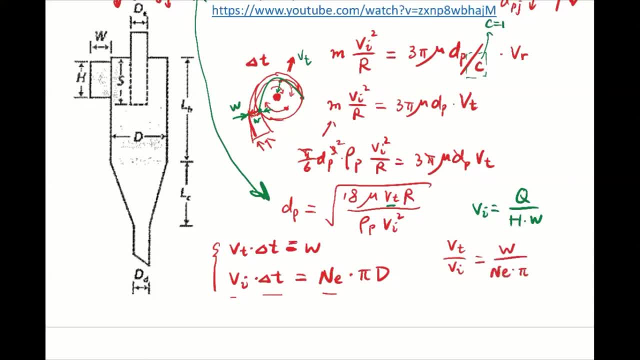 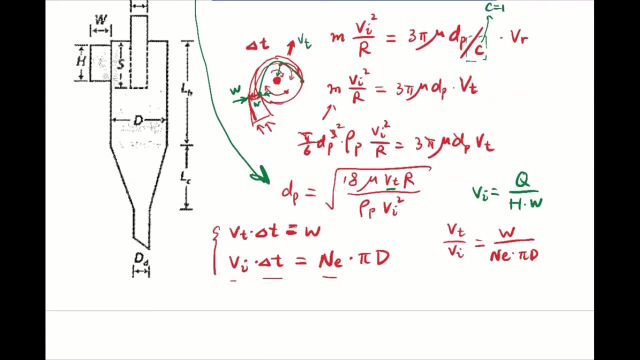 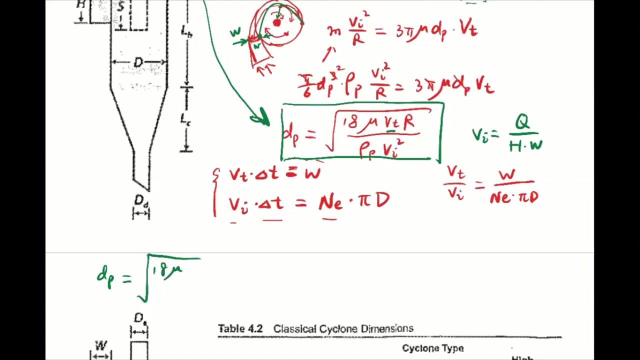 That's going to be w divided by Ne, pi, d. OK, So now let's look at this equation again. OK, So we have this equation right. I'll just put it here: dp equal to square root of 18 mu. 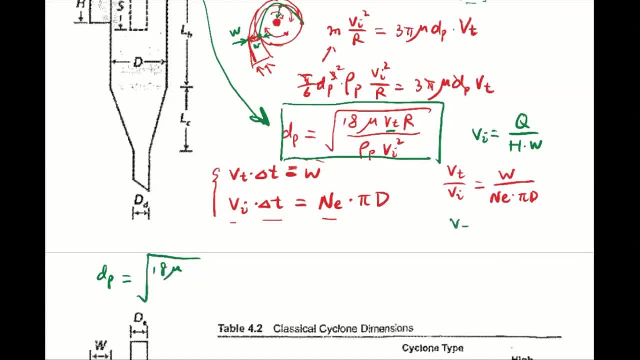 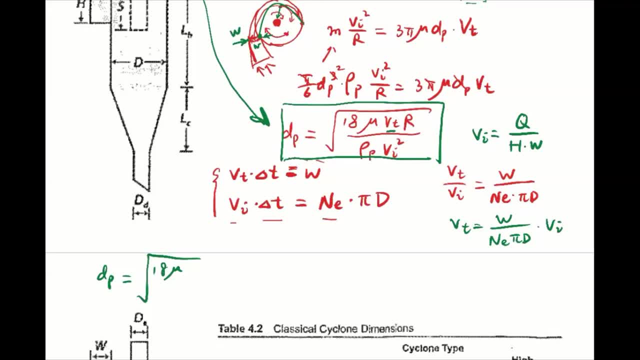 here w Vir divided by rho P Vi squared Ne pi d. OK, we can cancel a few terms. Vi and Vi can get canceled, right, Or it's just half of d, right, We have two here, so that's going to be equal to 9 mu W divided by Rho P VI PI. okay, so now if 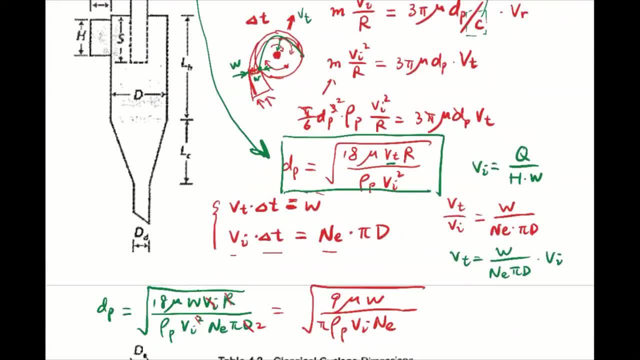 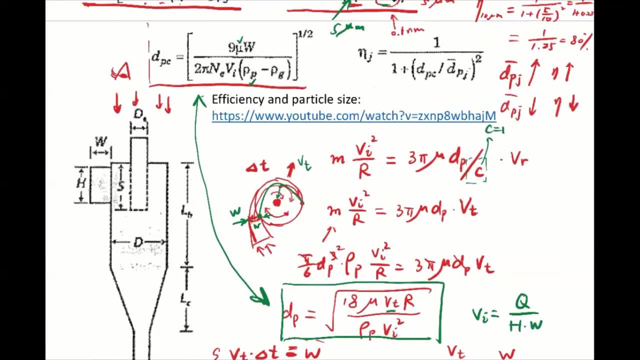 you compare these two equations. so this is what we have right and this is what's what people determined from the, from the simulation or from the experiments. okay, so you see that we have most of the terms ready. so 9 mu W- 9 mu W, we have. 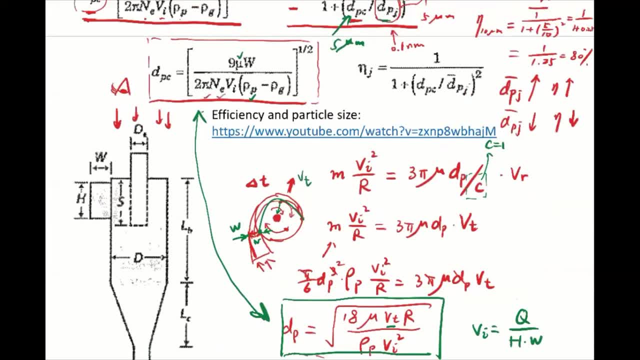 PI, NE, Rho, VI- all of these terms are ready. so finally, people decided that we need to put a 2 here to make it more accurate, but a square root of 1 over 2 is not. it's not a huge value, right, it's just a small modification. 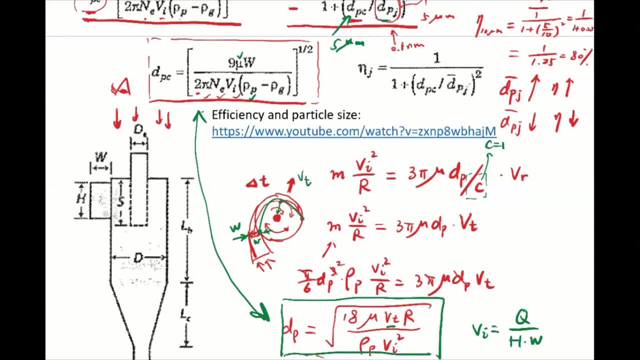 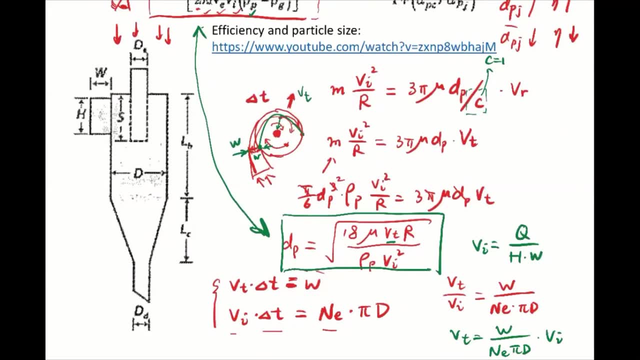 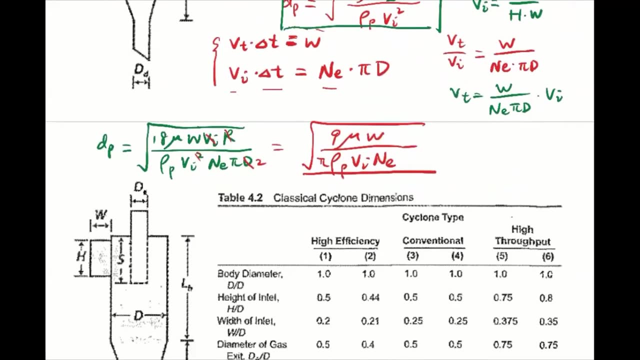 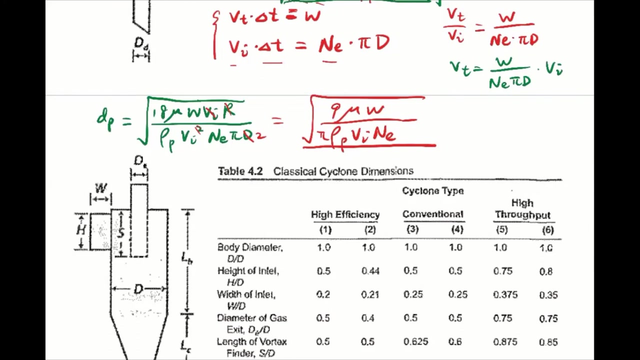 in terms of the, in terms of the final value. so now you can see, basically, by using the force analysis, by using the drag force, we can solve for what is a critical size of a particle in the cycle. okay, so in terms of the real design of the cycle or the real industrial application of the cyclones, people 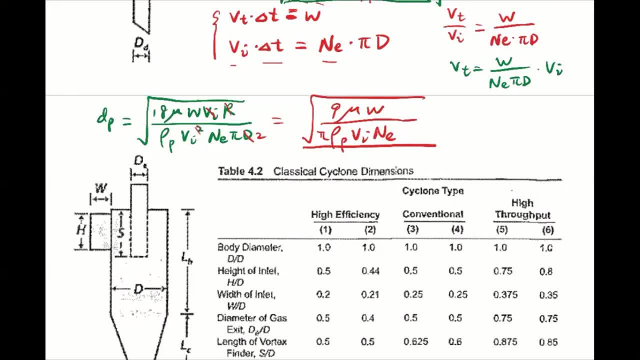 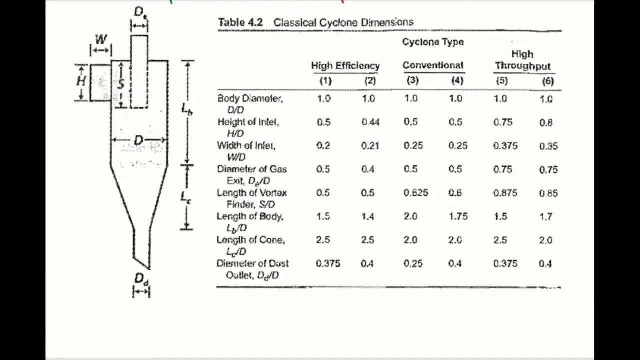 won't come up with their design randomly, so here is showing a table. so this is showing the classical cyclone dimensions, and people can choose whether they want high efficiency cyclones, conventional cyclones or high throughput cyclones. so high throughput cyclone just means that you have a high 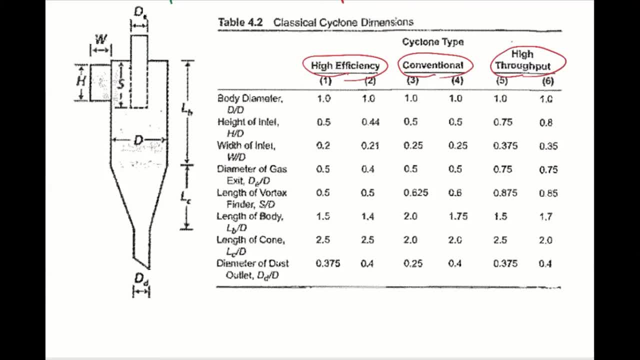 flue gas flow rate. the flow rate is too high so you have to let the air to go through at a high throughput right. so these ones will not have a high efficiency compared to these high efficiency ones, but most of the cases people will just use the 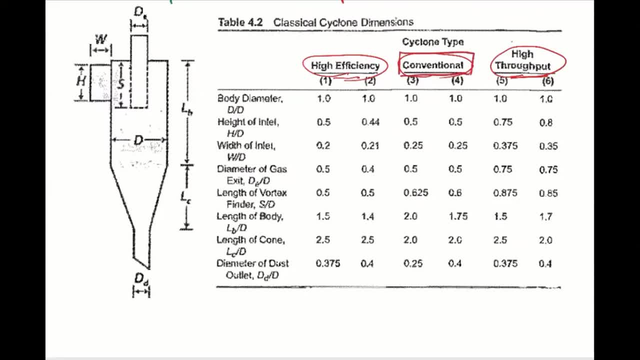 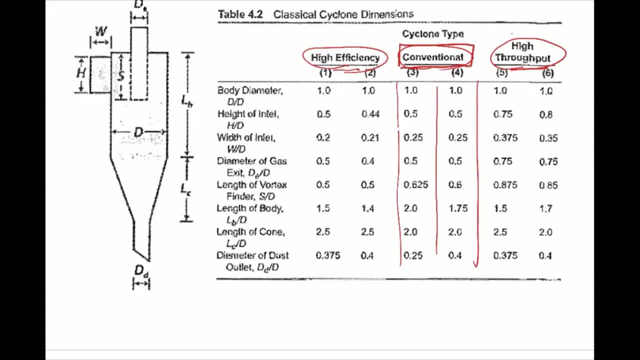 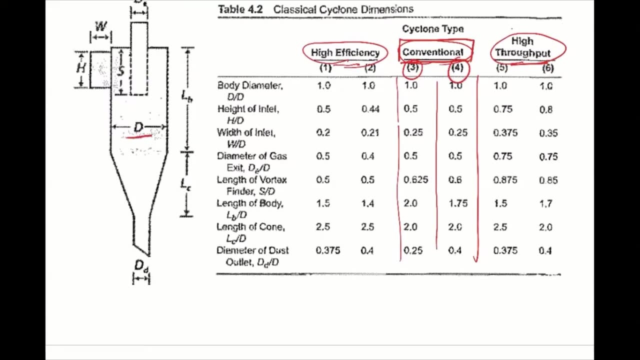 conventional design. so you can see that the conventional design is basically giving you a list of. so it's a three or four number. three or four, it's giving you a list of ratios that you can choose. so, for example, you decide that your diameter of the cyclone is one meter. okay, so then you can find out what is the. 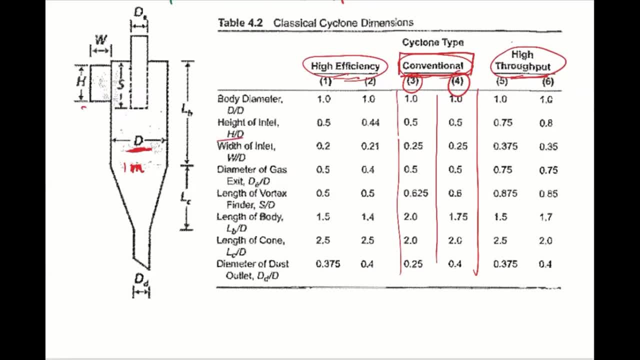 height of the inlet. so the H here right, H over D is point five. so the height can be 0.5 meters. right, the width of the inlet is 0.25, so that 0.25 meters. so everything is ratio or everything is non-dimensionalized by. 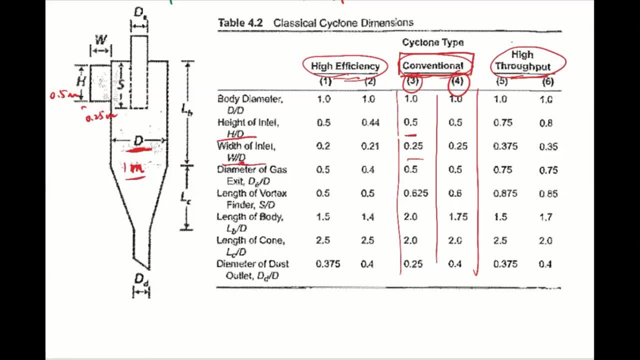 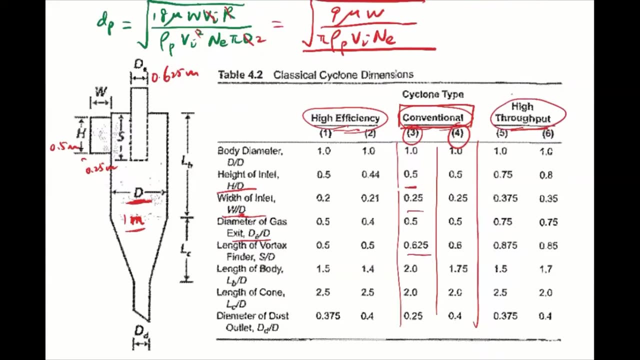 the body diameter, which was assumed to be one meter here, right, so the diameter of the gas exit. so here DE divided by D 0.625, so that's going to be 0.625 meters. right, it depends on what is the body diameter. if it's half a meter, then all the 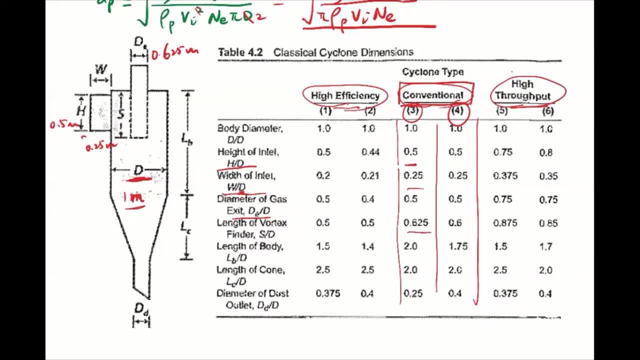 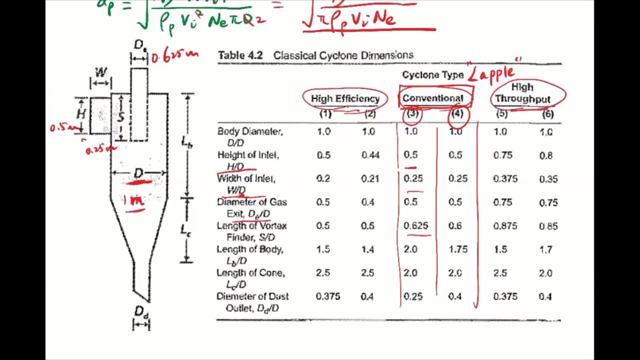 diameters will change. okay, so for this conventional type, people also call that as a lapel type, so it's just a name, right? he came up with this design for the cyclone here. so here we know that, once we know the dimension, and if we know the 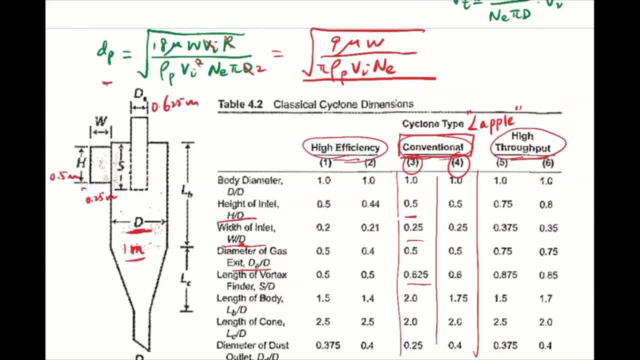 flow rate, we should be able to calculate what is the critical size, what is the cutoff size, right? we just need to know what is the air viscosity, right? the width of the inlet, the particle density, the inlet velocity. inlet velocity is just the flow rate divided by the cross-section area of the. 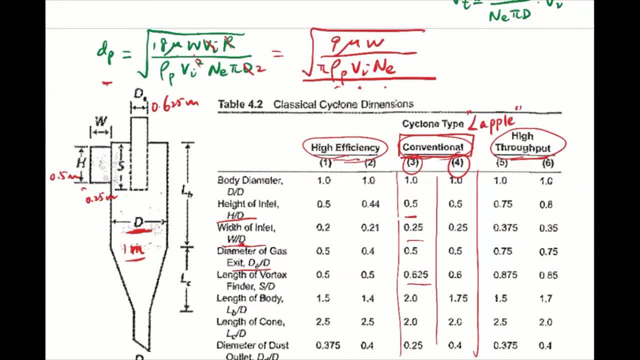 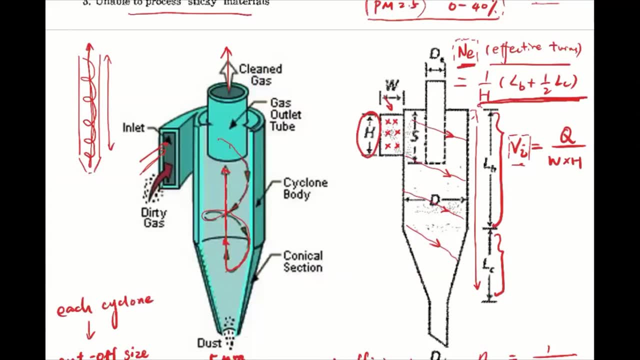 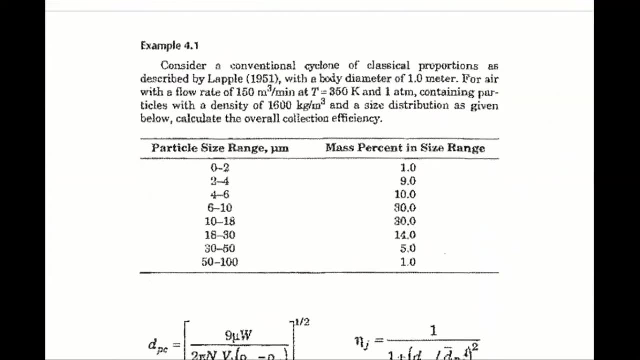 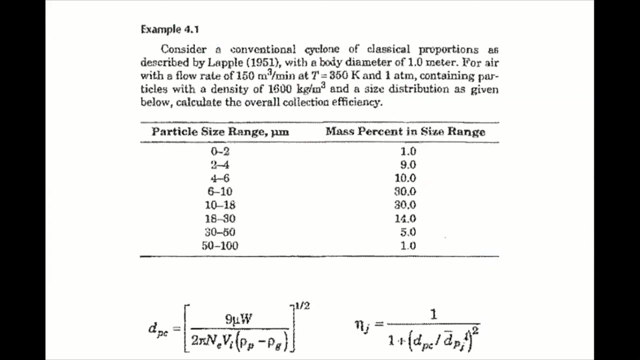 inlet, right, and the number of the effective turns. the number of effective turns, we already showed here, it's dependent on the cyclone dimensions, right. so with all of these parameters we can try to solve for what is the collection efficiency at different sizes. so this is an example, trying to look into what is a collection efficiency of particles of a.